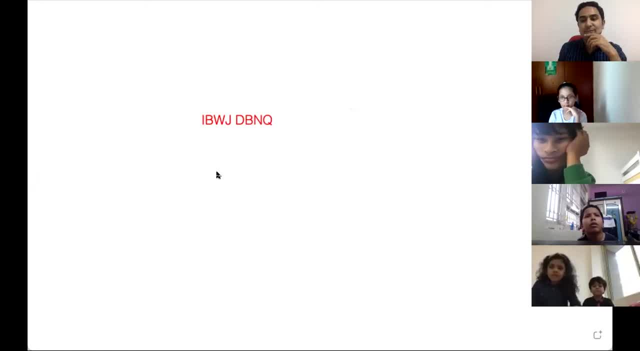 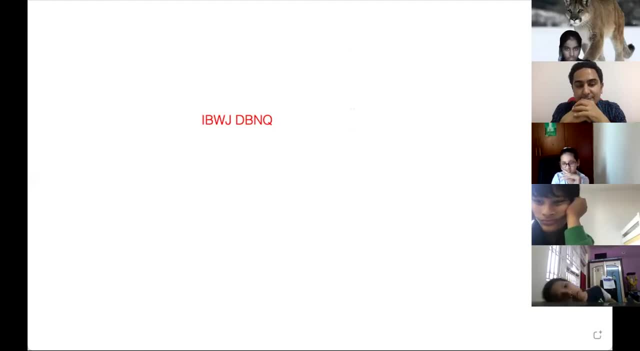 Okay, Can you now? can anyone tell me what's written? Okay, Can anyone? Yes, Arohi, It is written I, B, W, J, D, B, L, C. Okay, That's just A B C. I don't want A B C, I want the real thing, real word. How do you? 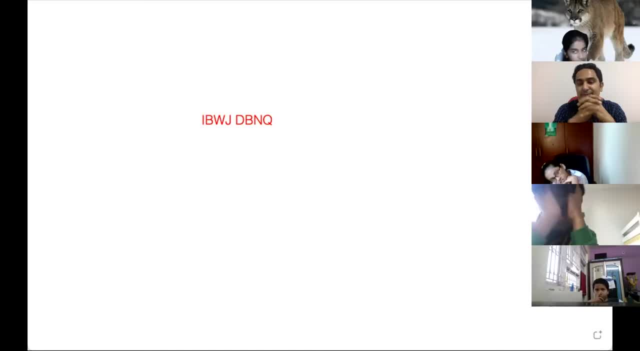 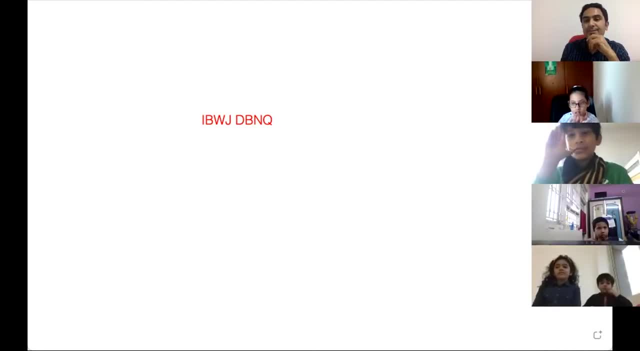 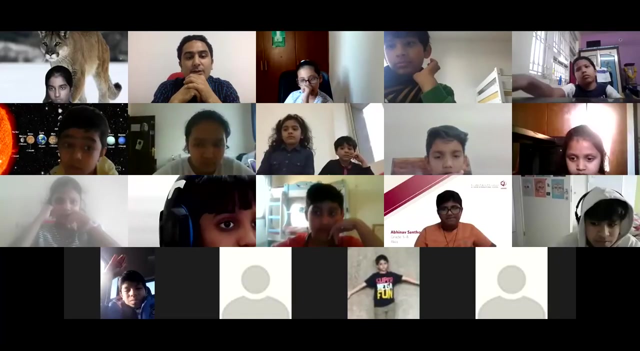 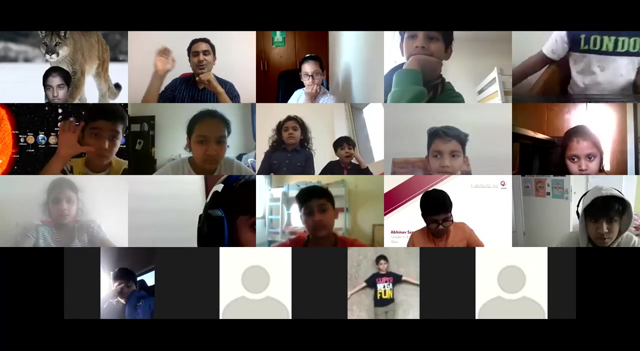 pronounce the words. Who can? Yes, Jainil, You did jumble the words, Jumble the word. Okay, Who can read this? Just a while back, you all say: know that you know reading. All of you raise your. 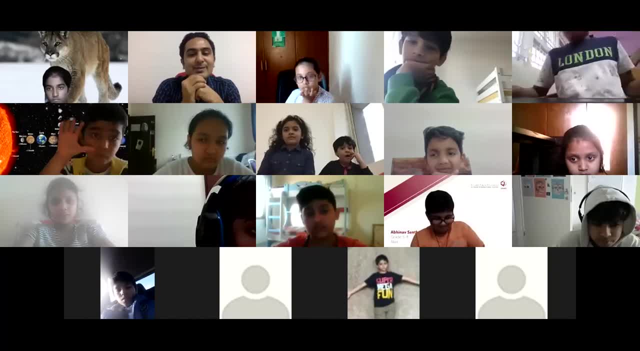 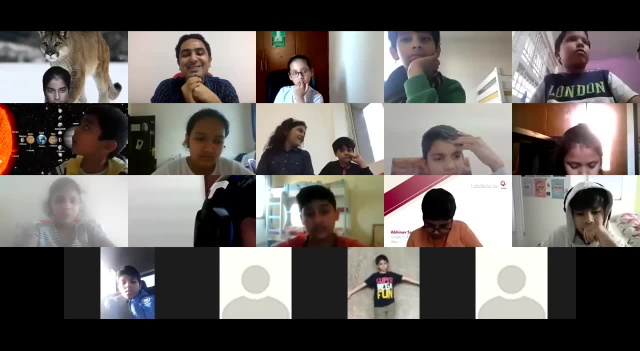 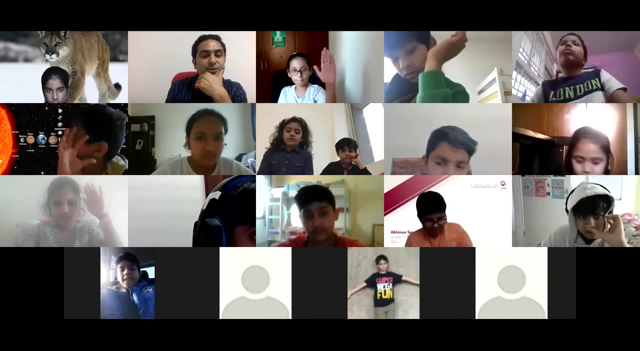 hand And now none of you have, you know, none of you is being able to read this out. How come? Hmm, So it's so strange, you know. let me tell you one thing. Oh, okay, Sarika wants to say something, It seems. Yes, Sarika. 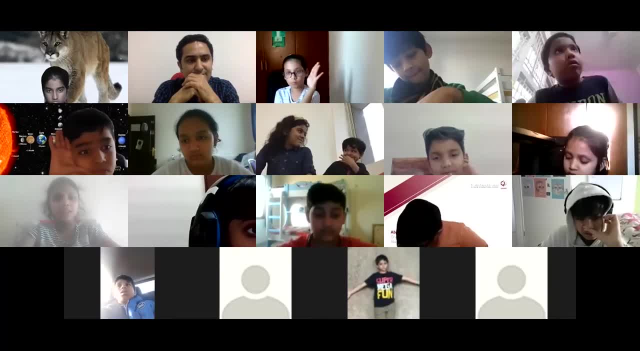 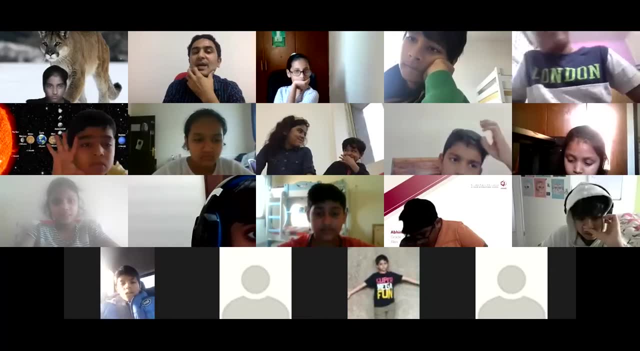 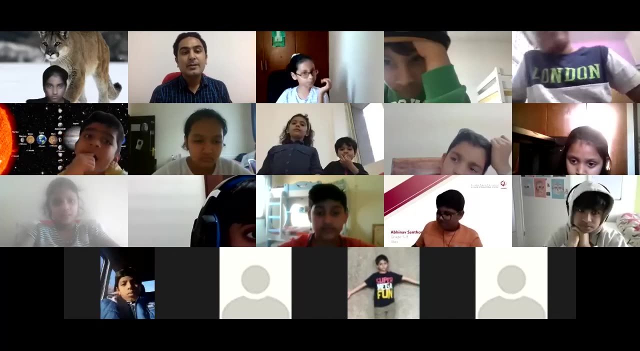 Sir, we did not. we were not able to pronounce it because the word was unfamiliar. Okay, The words were unfamiliar, Okay, Nice. Good explanation, Sarika. So let me tell you what you know. there is a spy. 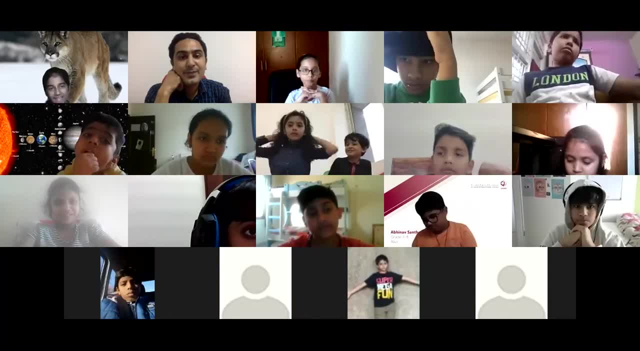 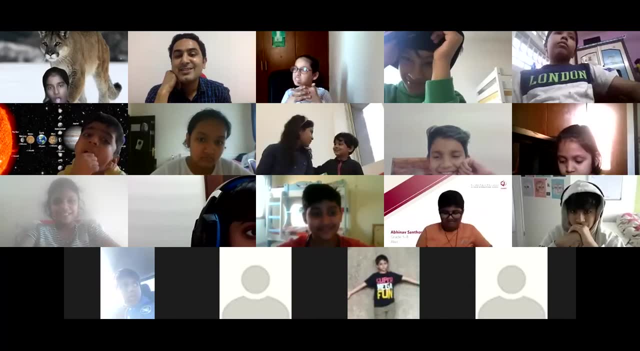 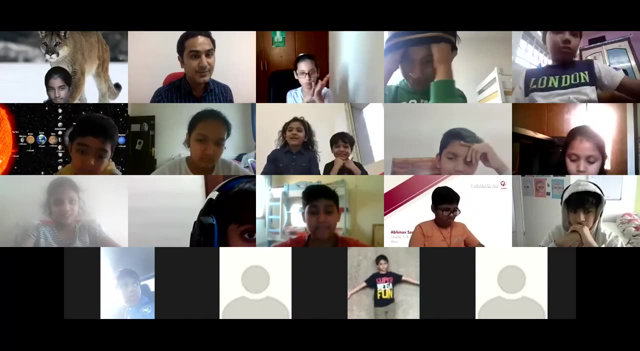 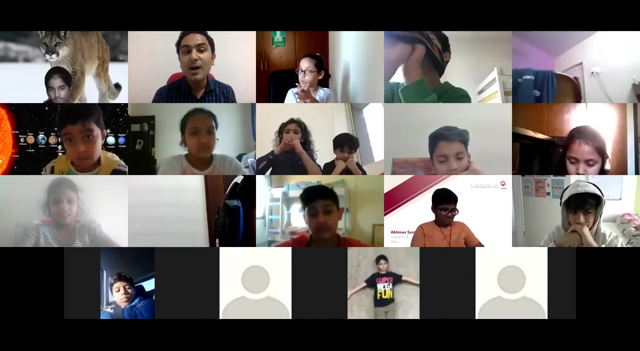 Yes, a little spy. His name is Jassus Chintu- Yes, Jassus Chintu. And Jassus Chintu got some very secret information. Yes, some very secret information. The information was you know were all about. 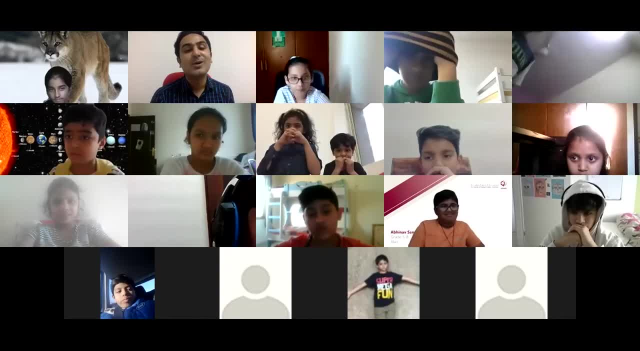 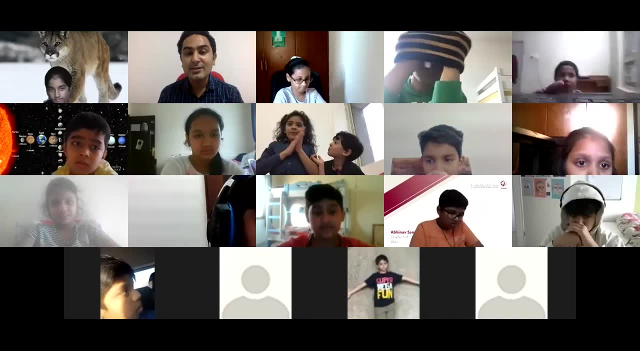 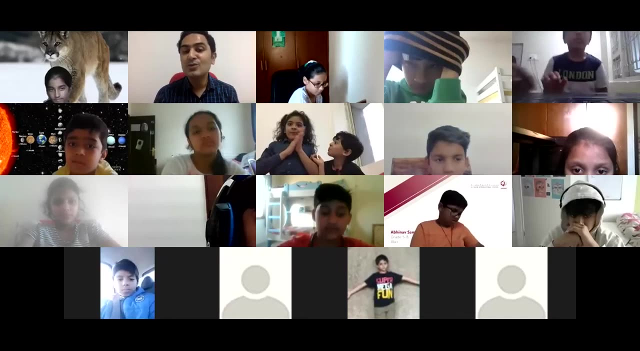 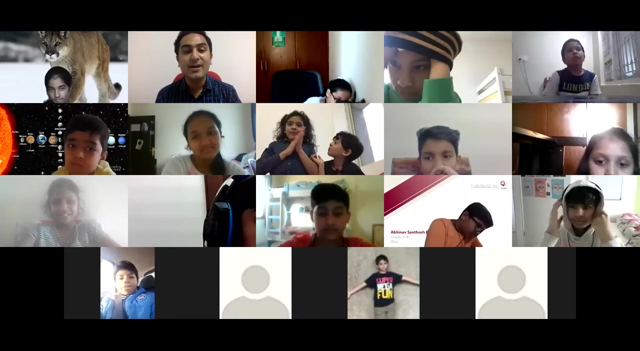 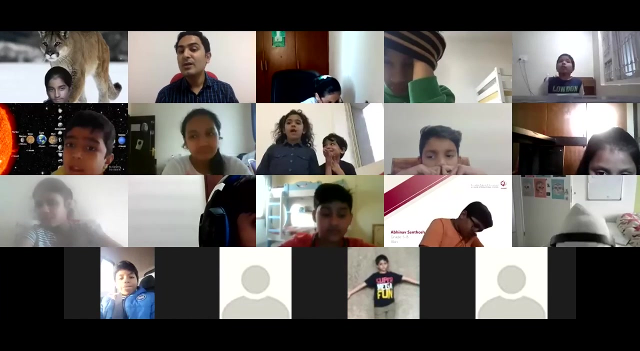 where the the ice cream is stored. no one knew about that, so jasus chintu found that out and he wanted to tell this to his sister. her name was jasus chinki, so jasus chintu wanted to communicate that to jasus chinki. that where where this ice cream is stored. but if he sees out that loudly, 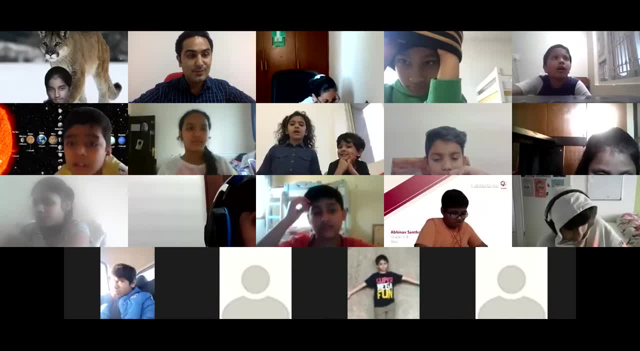 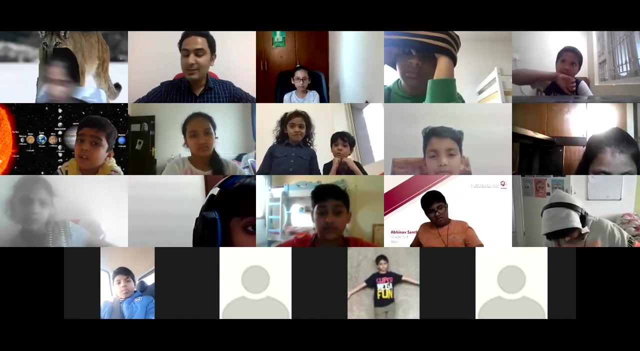 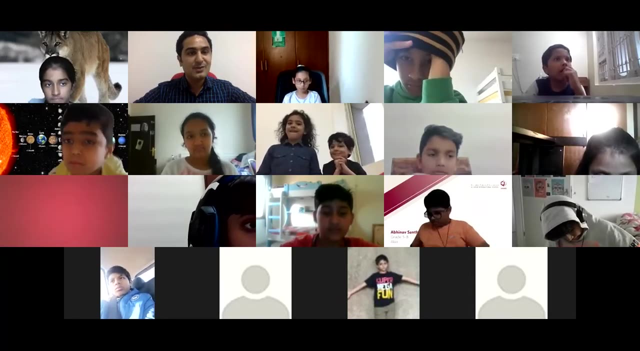 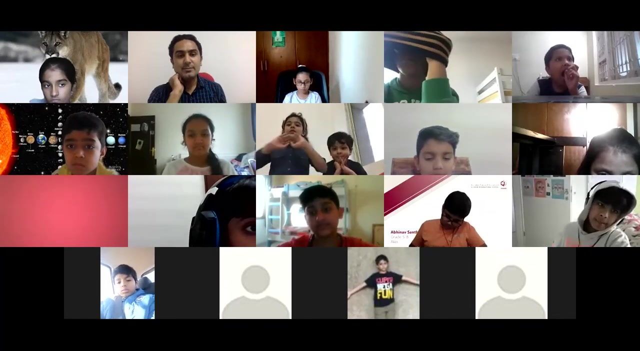 and everyone other, every other one would know and will come to have a share of the ice cream. or the parents would say no, no, no, no ice cream. at present it's the viral infection season, so no ice cream. now what to do? he wanted to say that, so one way is. there is one way. one way is as, like anaya, 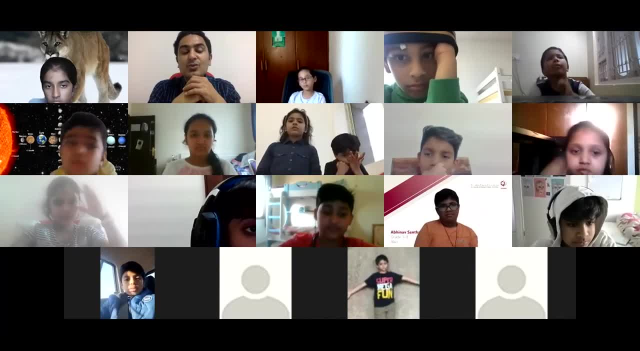 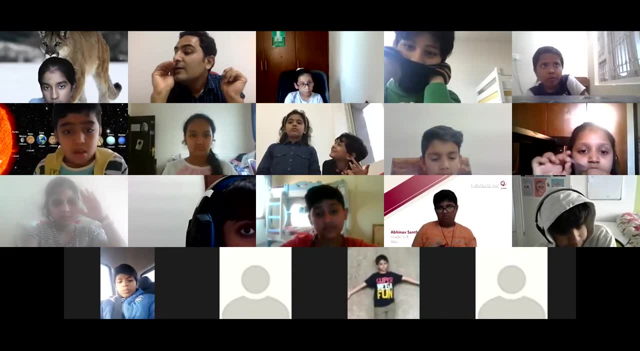 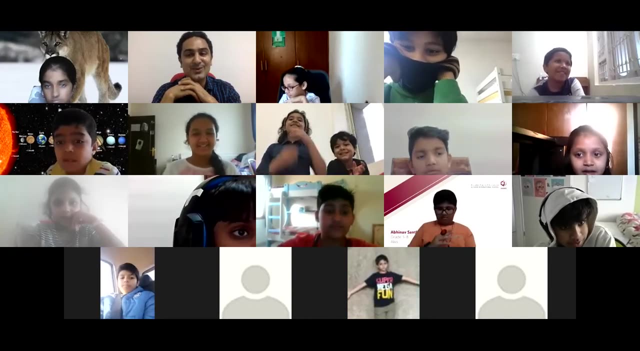 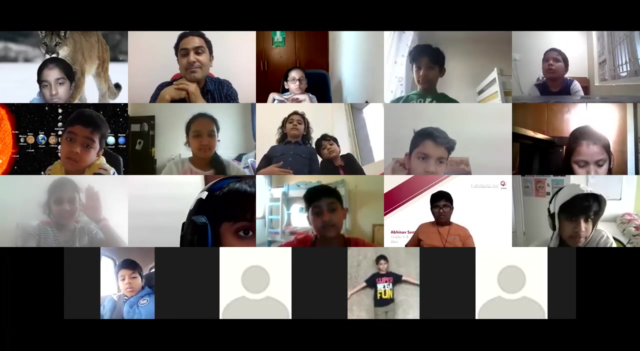 and havisha are sitting together. the chintu can go near to the ear of chinki, jasus chinki, and say like this: yes, that is one way, isn't it? or no? then no one would know. but what if they are at distance? What if they are at distance? Yes, Sarika. 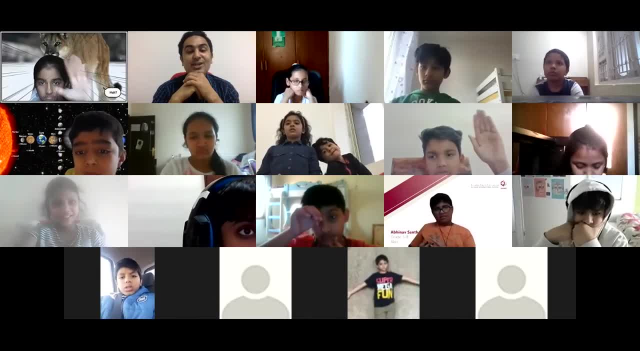 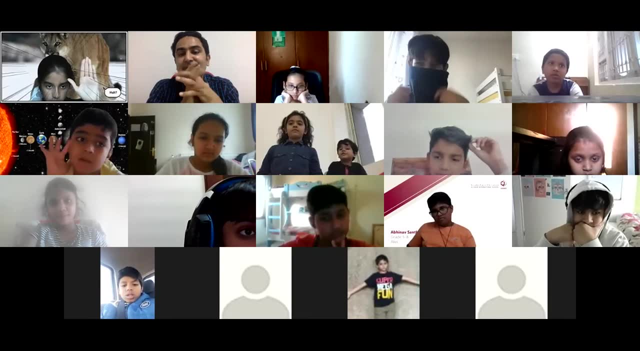 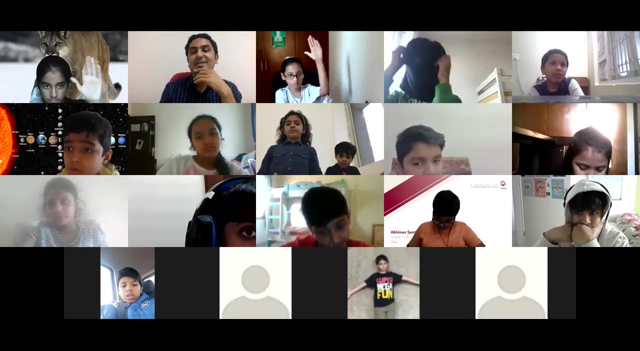 Sir, they could use a secret code, Secret code, yes, What that secret code would be? Yes, Aarav, Sir, they can use a code language, Code language. What code language? How You know? like A stands for one. so like that, Yes, Yes, Aarav. 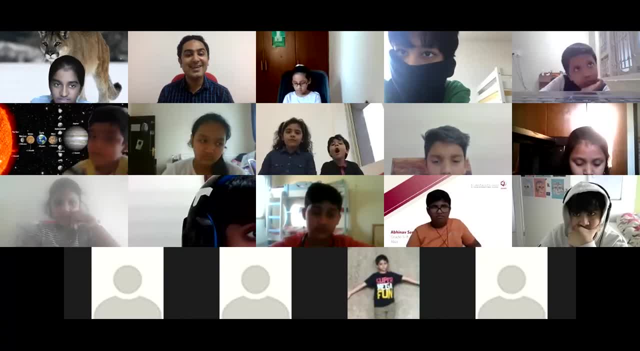 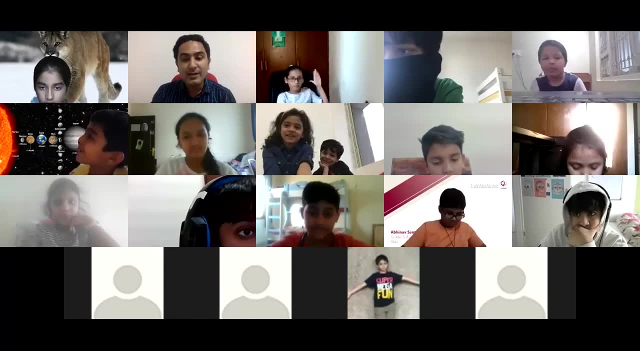 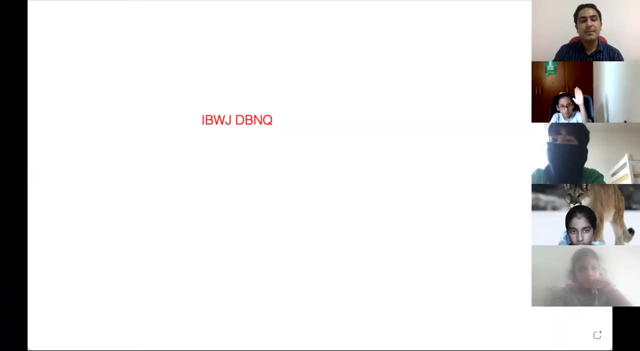 Sir, they can use walkie-talkies. They can use walkie-talkies, yes, Possible. So there are. you know, these are all the ways, and one way I will share my screen now See what is a possibility, If I want to say something like: 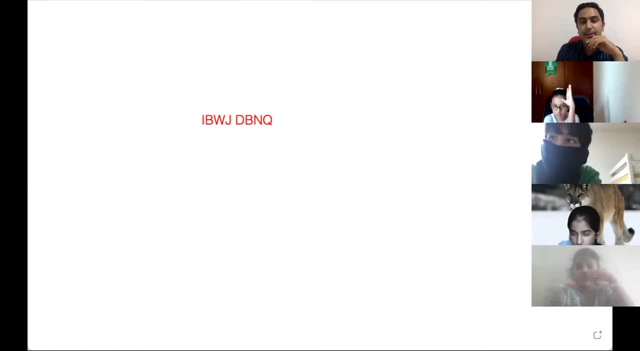 like: okay, I will type it here: Ice cream is in box number four. Okay, Now can everyone, can every of you, read this? Yes, box number four, right Now. the thing is, they don't want to communicate this as it is. 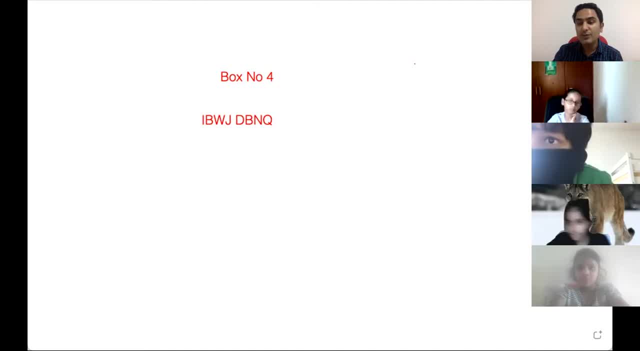 Yes. So what will they do? I will show you What did they do. See, here I am going to write the entire A, B C D. Okay. So A B C D, Okay. So here is the entire A B C D. Now what will they? what you know this. 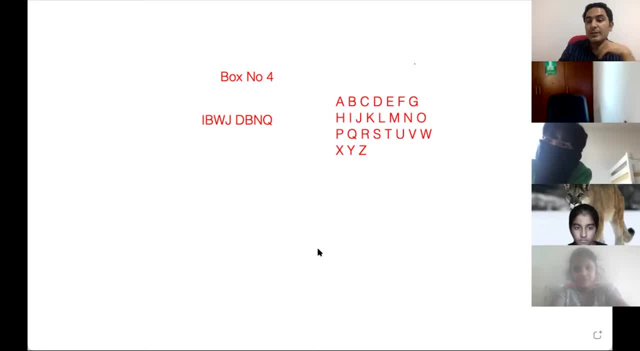 Jassu's Chintu did What he did. He used the B, So where is the? this is the first character, That is B. And then what he did. He added one into that. So what comes after B? What? 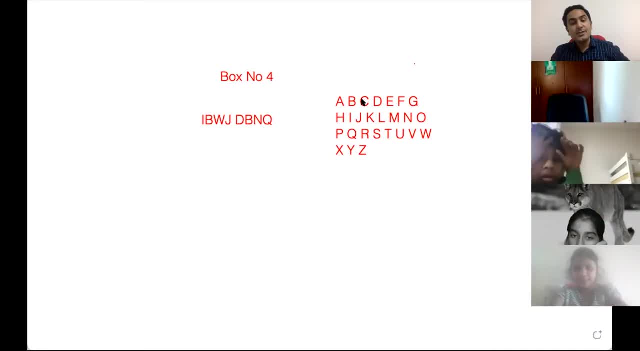 comes after B, C, Right. So what he did now, He wrote C. Okay, He wrote here, instead of B, he wrote C. Then, what comes after O, It's P, And what comes after X, Y, What comes after N, O, And. 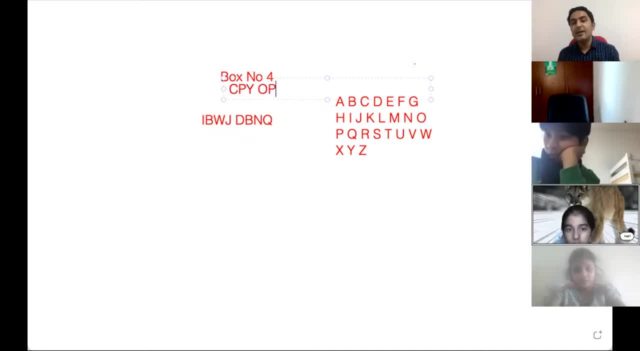 after O It's again P, And then four. let's consider four as it is. So C, P, Y, O, P O R O N, And know after answer: A, B, C, D, O, M, V, Y, O, T, L, O, P, G, So five sets. 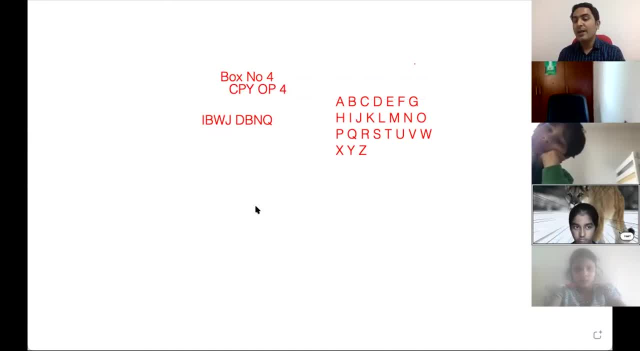 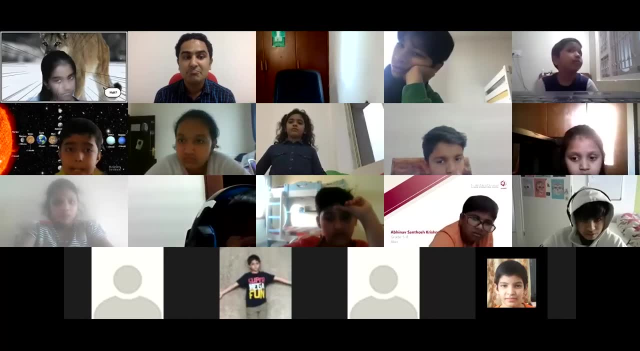 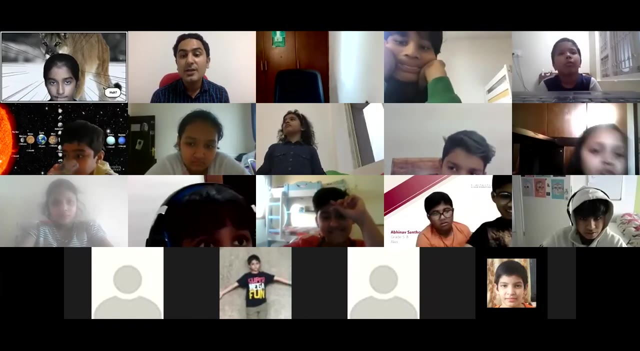 of aside. einmal B after O, B, Q, Y, O, M, N, So that's O with N, so it comes after a Colonel. And then when is it clear? So twice here. and what comes after B, C, D, So this line there again. 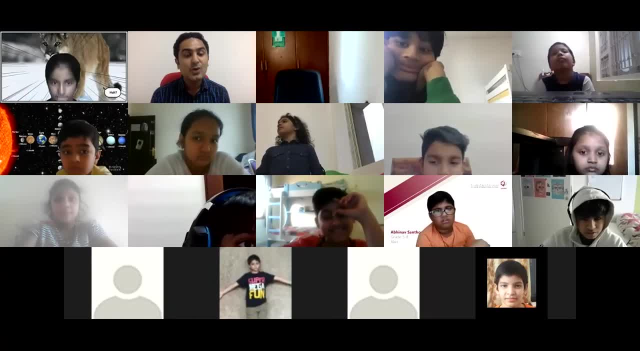 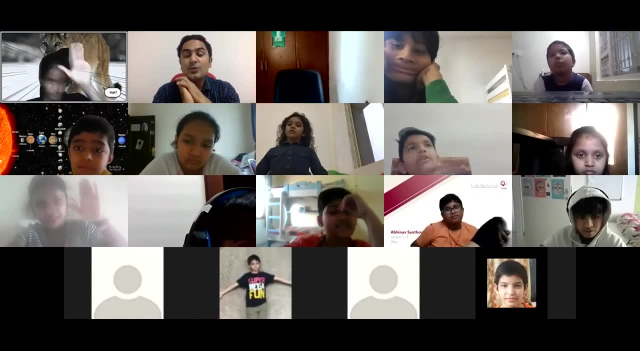 ��요. they have aippy line with you Forever there, over and over. I am marking this. So the first line here comes here, in four verses: B, Q, L, M, A, T. So when I sprinkle a couple, 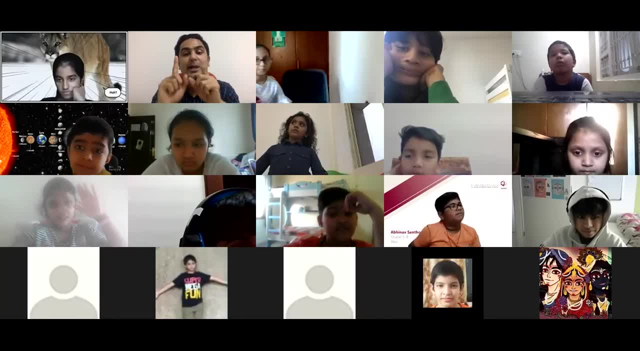 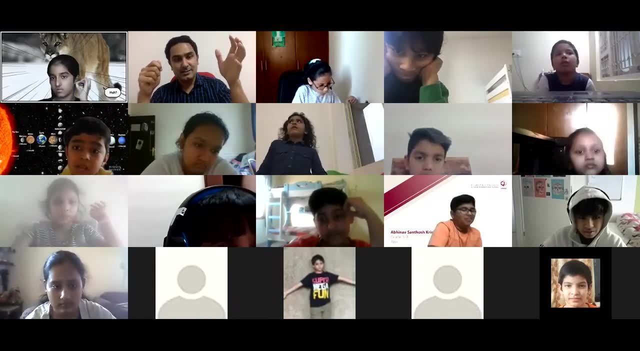 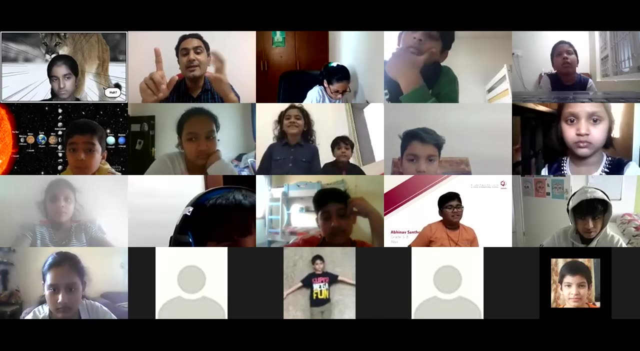 down, it becomes T. Now I am not writing down which language is implemented in this, So that what they need to do they'll have to decide a key, one key. they'll decide one key. so you know, this text is a lock and a lock can be opened with only one key. so they will decide a key that our 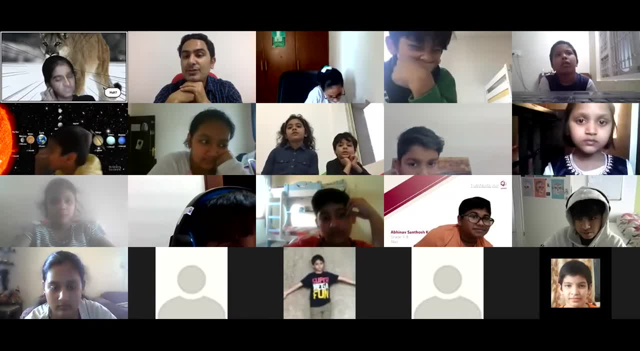 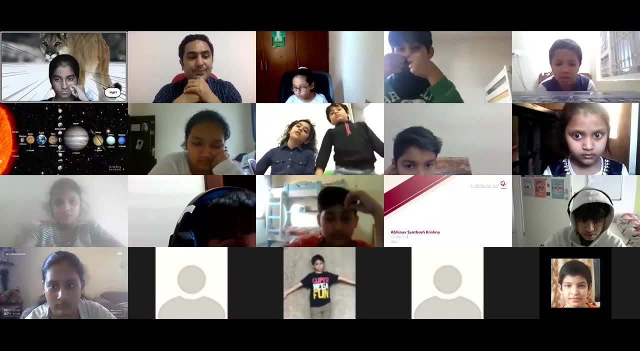 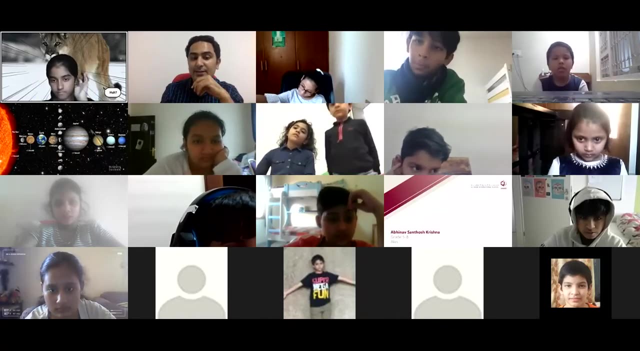 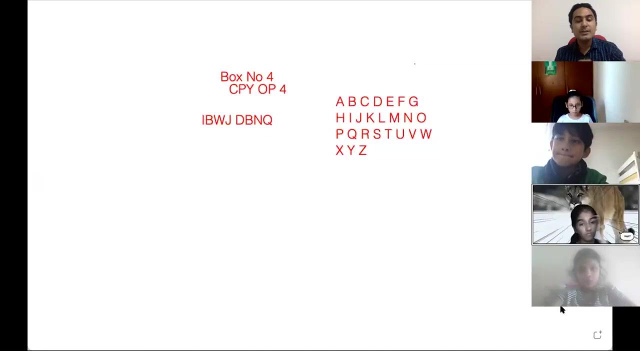 message. how will we unlock our message? let's decide one key, and that key is what that key is: number one, am i right? number one is the key. so now, when jasus chinky receives that this message, i'll share the screen again. so when the jasus chinky receives the message, what will she do? 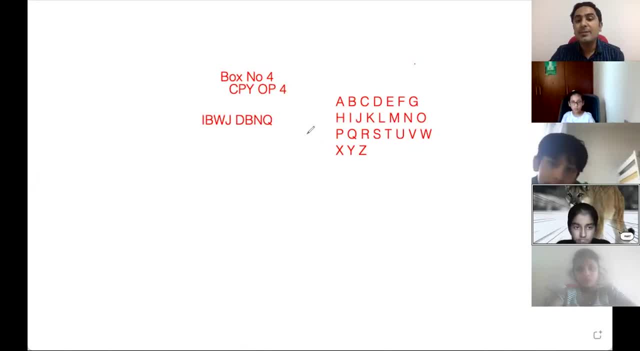 she will use the key and will be that. that means what comes before c, the v, what comes before o, i'm sorry, what comes before p, that is o, what comes before y, x, then o, n, p, o and four. so that is the key. now, what will they do next time? they will change the key instead of one. now they will. 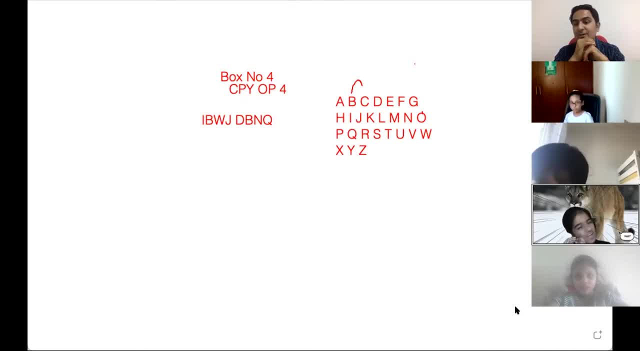 use two as the key. will that work? okay? okay, yes, that will work, they will use two. so instead of now, next character, they will jump by two. so in that case, what will happen here? instead of now, b, b plus two, what is b plus two? d, right, b plus two is d. b plus two, that is d. 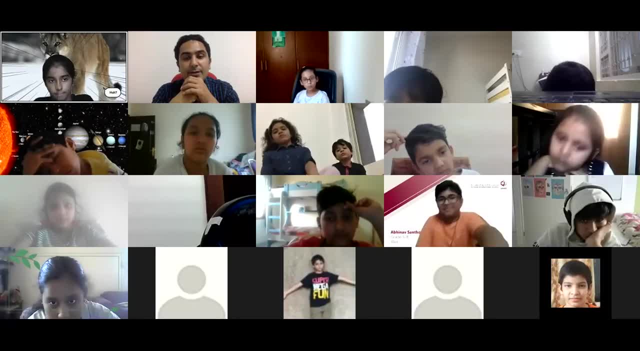 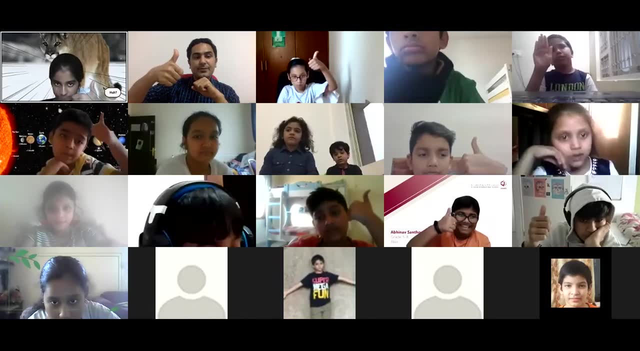 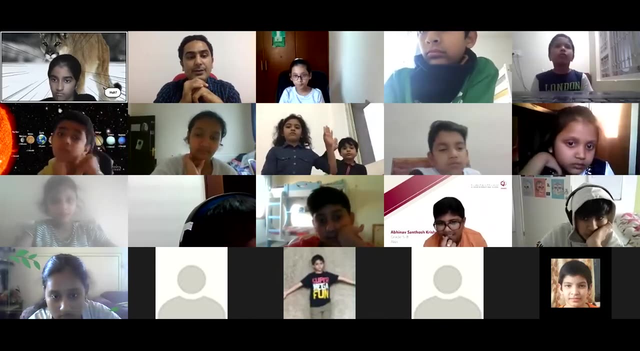 are you all understanding this or any question? all of you understood? show me your hand. can you show me your thumb if you understood this? okay, who is who doesn't understand? wouldn't understand. show me your hand if you don't understand. yeah, havisha, okay, fine, so avisha. uh, what are we doing? is we are adding. we are adding. 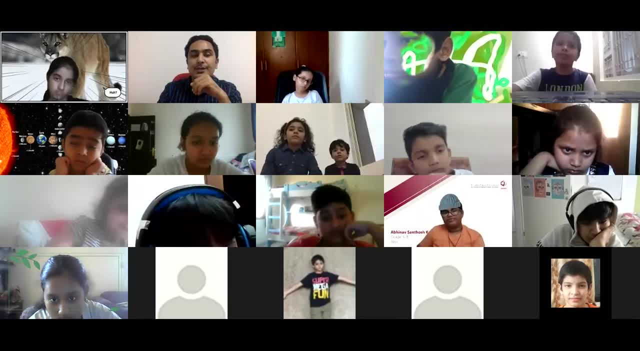 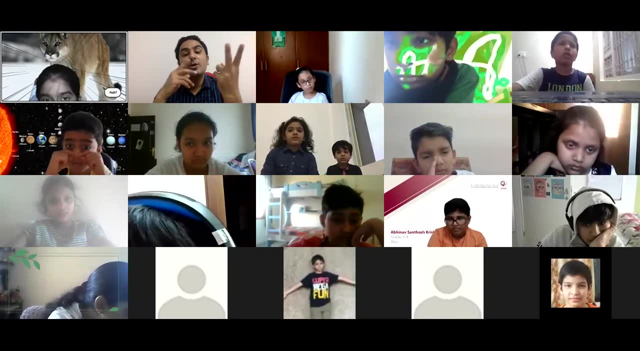 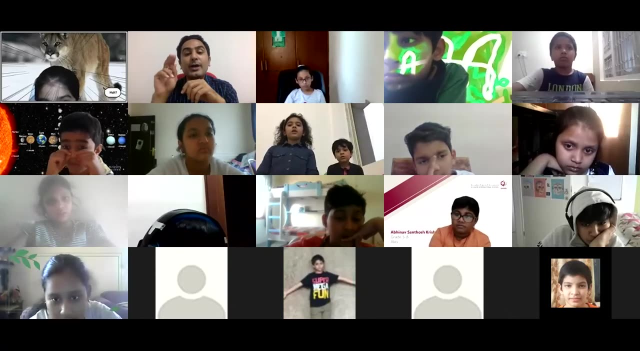 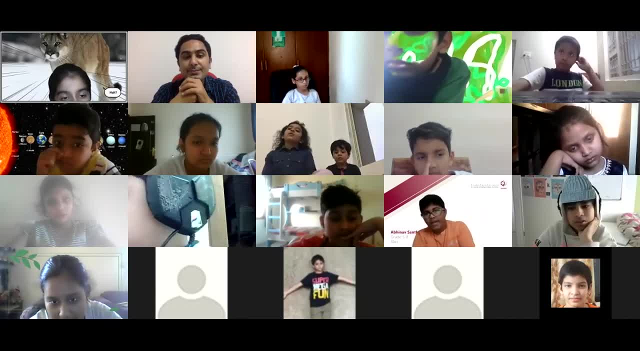 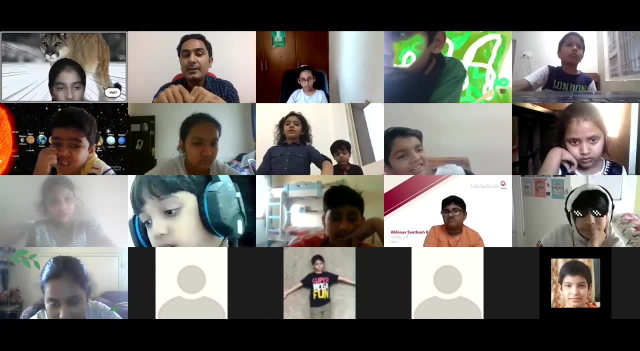 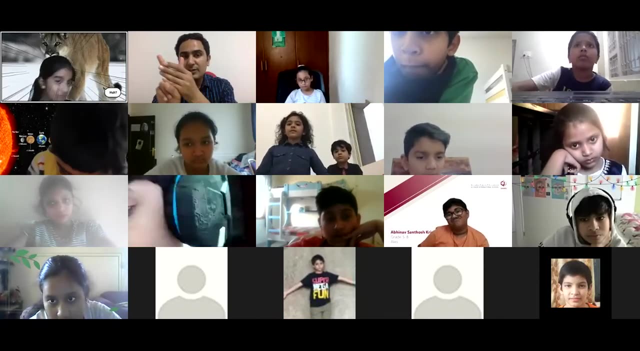 b, yes, b. what is the position of b in alphabet? second, huh, second, very good. so, number, what is the number of b? that is two, am i right? right? so now to add: this is two. now you add three into this. what is the total? two plus three? 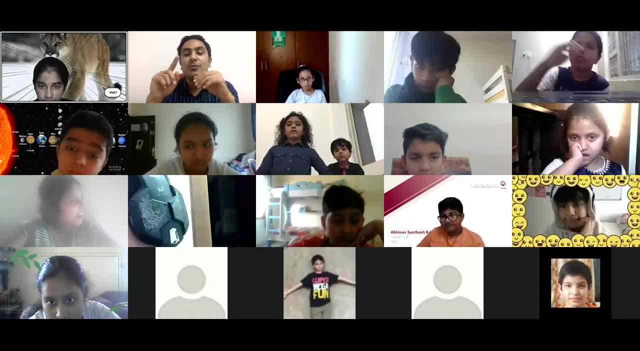 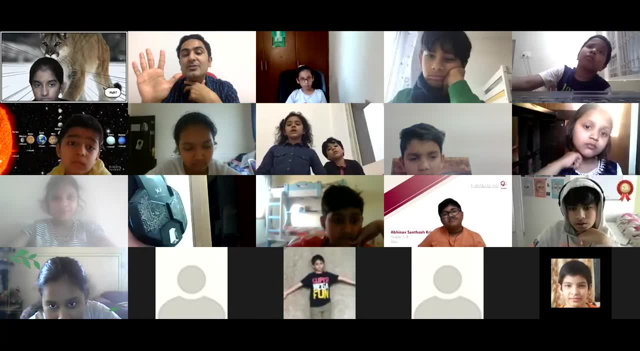 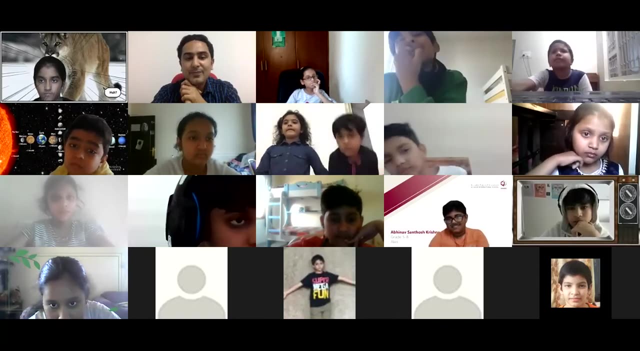 five, very good, now five. can you tell me which is the fifth, character K, which is huh very good. so now you replace b with e, is that fine? and that's what we have to do with e. so now you replace b with e, is that fine? so this is what we. 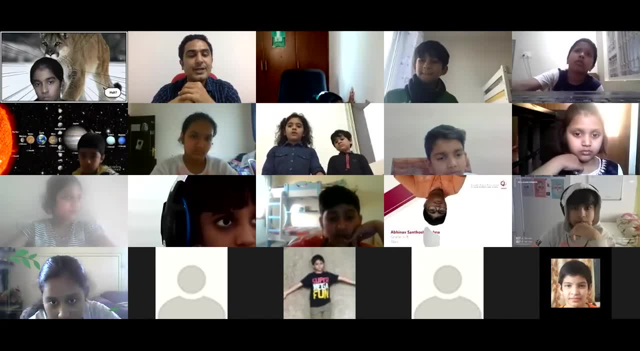 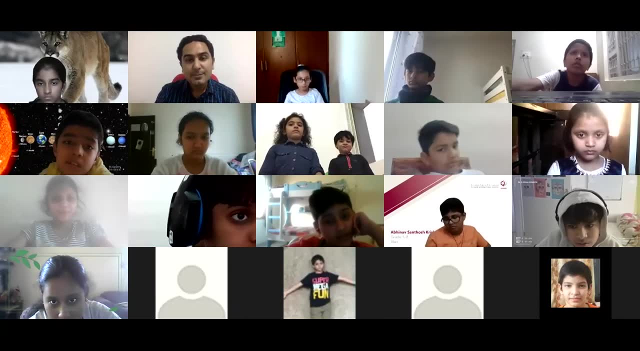 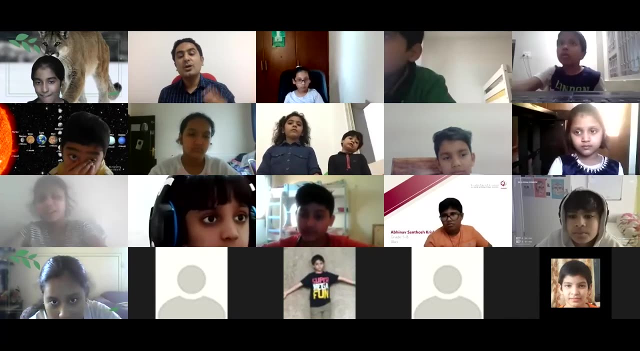 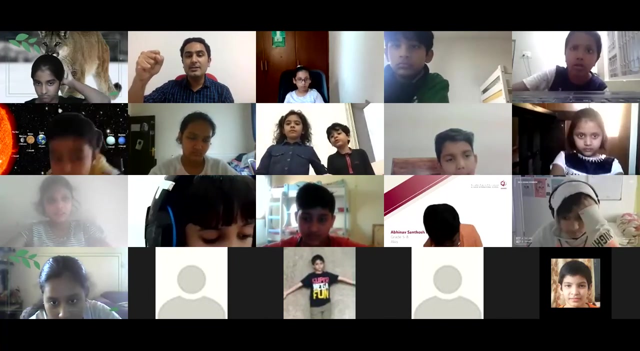 is what we are doing. understood now. very good, all of you. okay, so this is called key. this number is key. you need to know that key if you want to unlock the message. so on one side, when you have the key, you lock the message and you send the message and here the destination, you use the key. 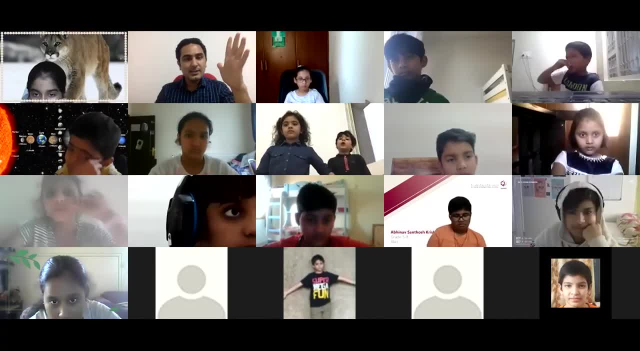 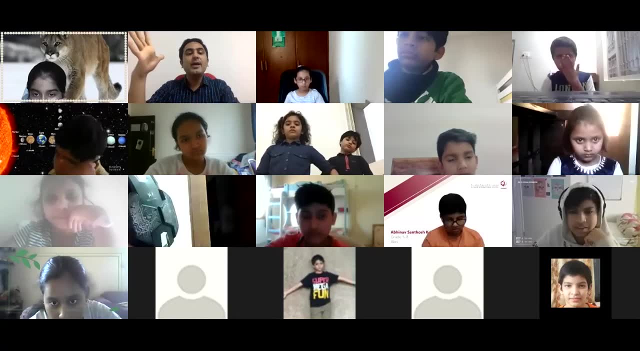 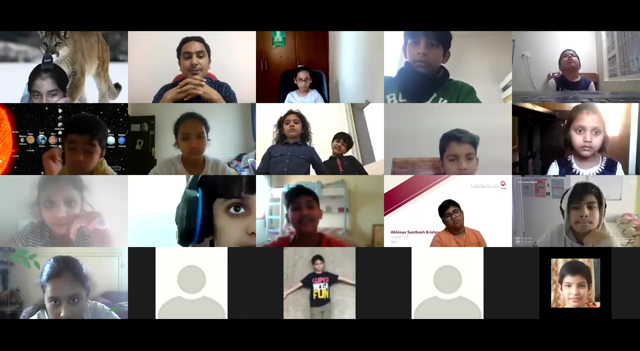 and unlock the message one more time. this is the message. you put a key and you lock it. you send the message here. you put the key and unlock the message. the message is open for you. so this secret message is being passed. no one else in between will know about it. okay, this message. 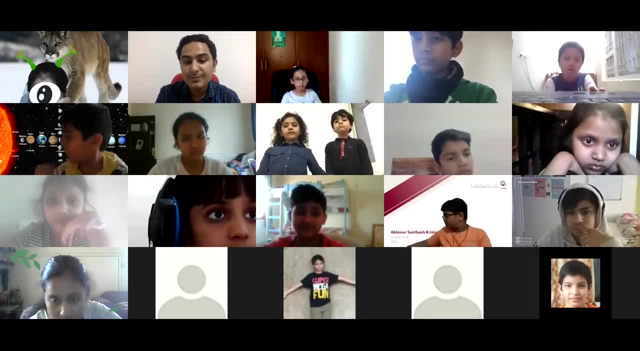 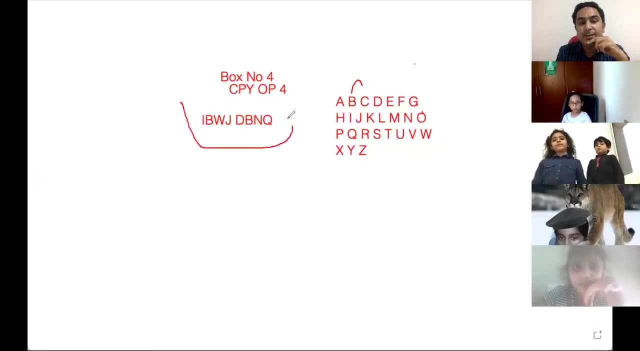 the very first text which i shared with you. uh, this one. can you now tell me what is written in this? the key is one, the key is one. you, what you need to do, you need to deduct, remove one from the first collector, one from the second character and find out what is written. 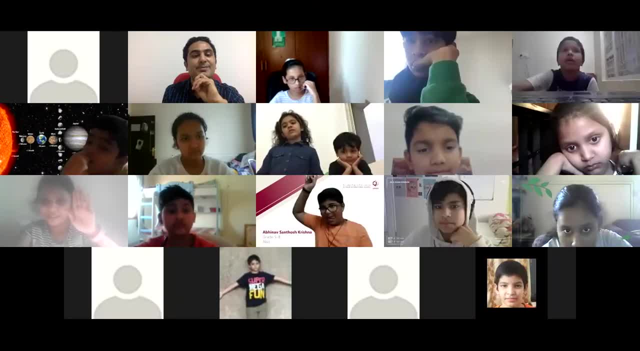 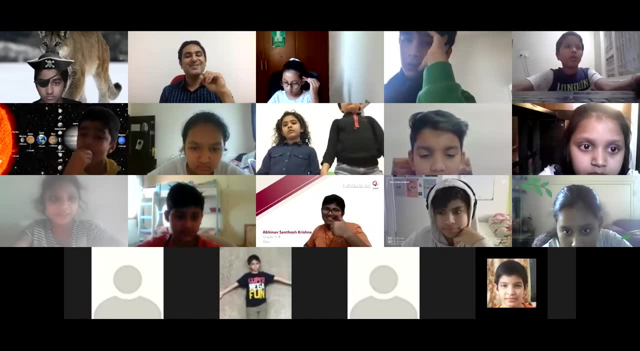 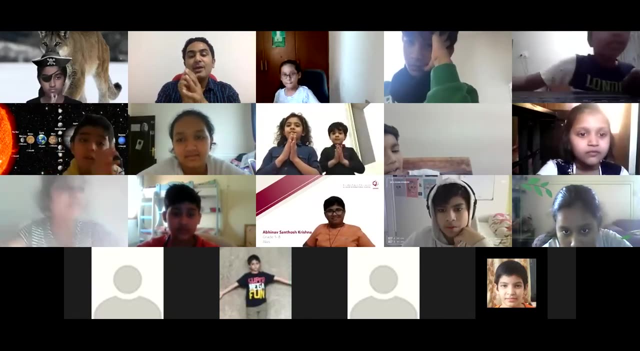 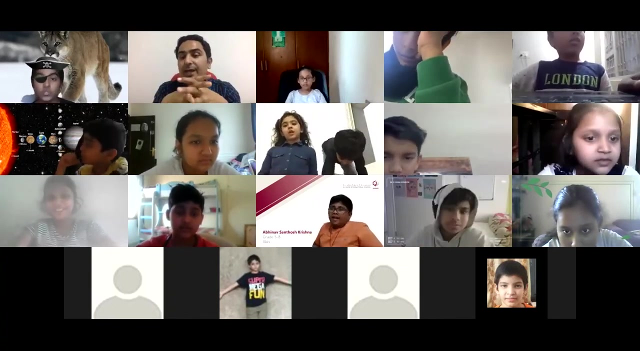 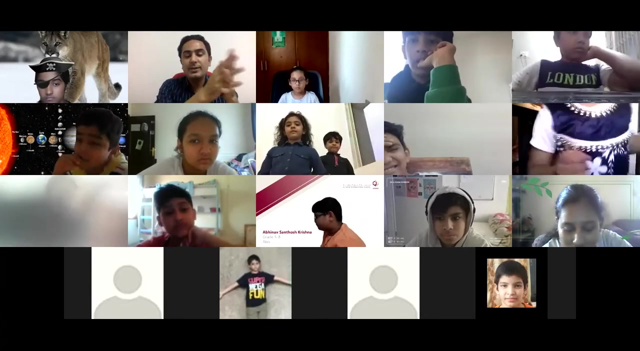 fastest fingers first. yeah, sarika, how we come. yes, it was written. how we can. nice clap for you, sorry. good, so this is called cryptography. what we just did know a way to sign the secret message from one way to another, one destination to one, in a source to destination, one place to another place. 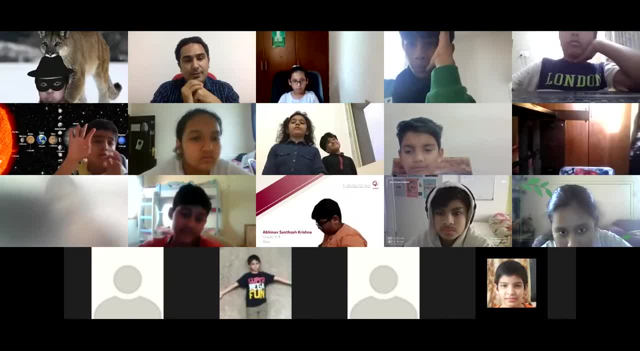 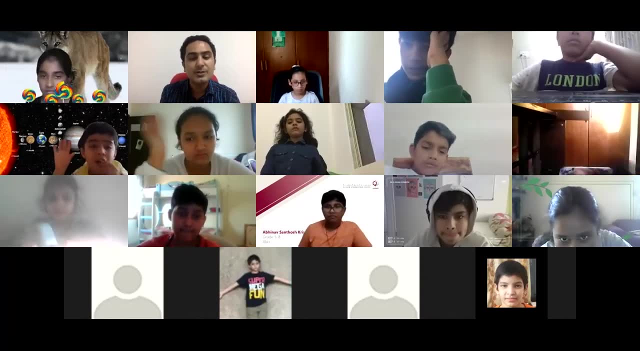 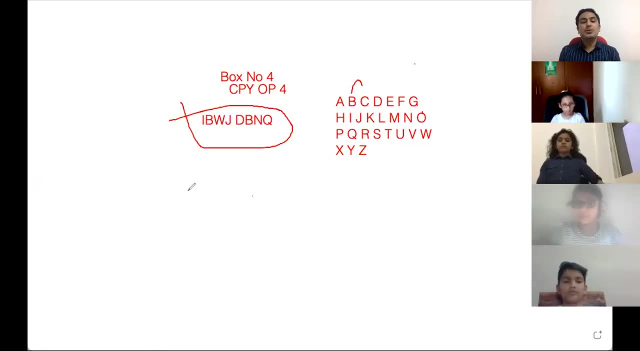 it is called cryptography. you understood that cryptography is the word. there are some words which, if you you know, try to remember these words. i'll write those so you can refer this back. so one word is cryptography, okay. another word is cipher text. another word is plain text. now, plain text means our original. 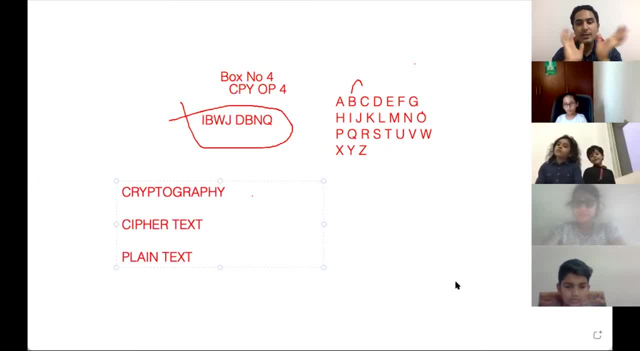 message, okay, the original message. and cipher text means this kind of message, the secret message. it is called encryption, this process converting plain text to cipher text, that is called encryption, and then converting cipher text back to plain text, that is called decryption. okay, so these are the words. cryptography: that means sending secret messages from one place to 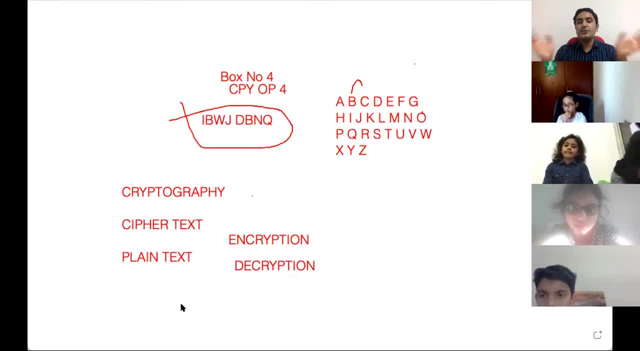 another place. that is the entire stuff. that is the whole thing called cryptography. cipher text, that is this coded message and plain text. that means plain message. encryption means converting your plain text to cipher text and decryption means reverse cipher text to plain text, and the last word is key. 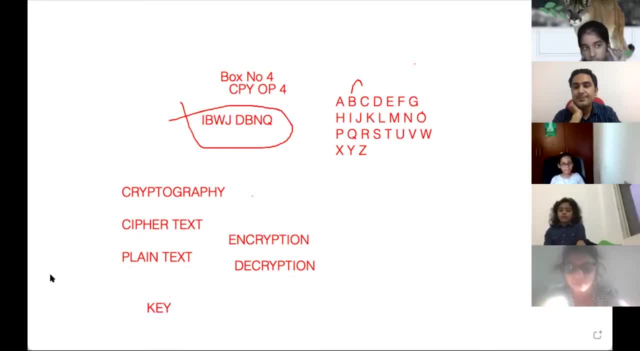 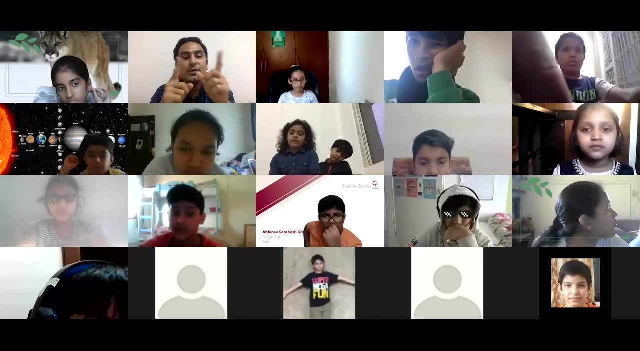 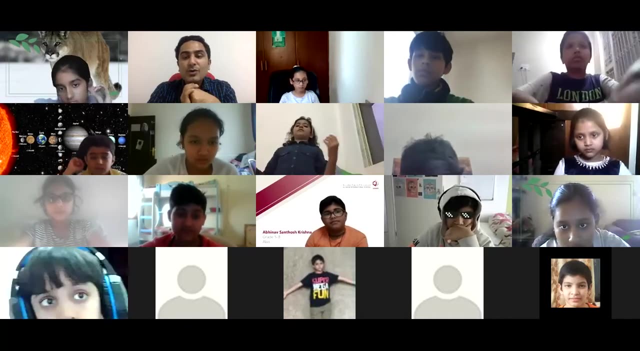 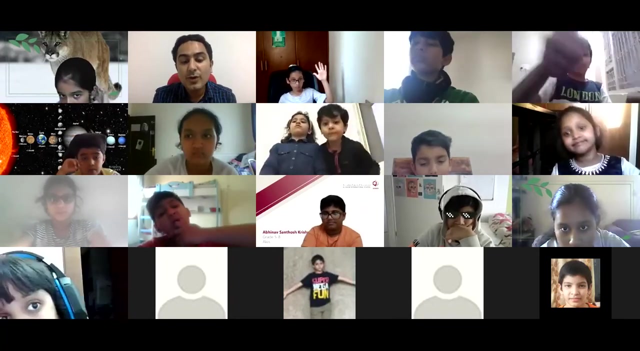 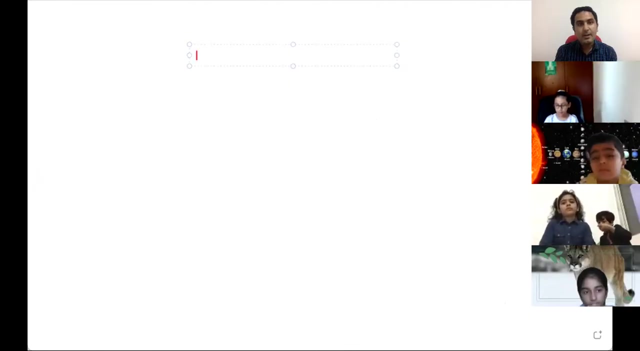 key. okay, key, we can use this and create our own, our own encrypted messages. okay, now do you all want to try this yourself? yes, so what i do now is i will write something on my screen: i love k�들by. okay, this is the message. now convert this into cipher text. this is plain text. 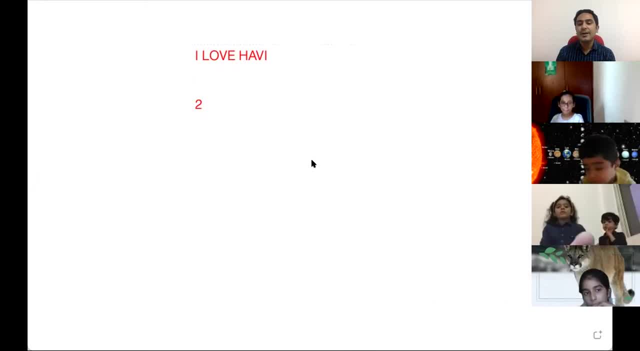 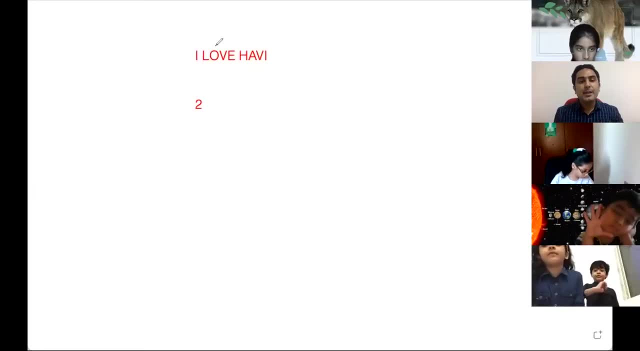 your key is two. okay, let's, let's do this. okay, shall we? okay? now, as we know our message, our plain text is: i love duke Howie, and our key is 2.. Now let's start coding this message. For reference, let me write ABCD. 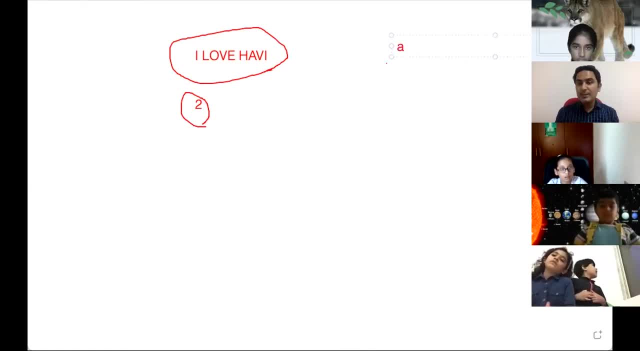 one more time. See, I am writing ABCD twice in a day. That's a shame, right? I have to write ABCD alphabets twice in a day. That is my homework, ABCDEF. OK, so this is the ABCD. Now our key is 2. so we will write it. they're starting going, So let me go back and fix it. Let's see if I make it. This will issues 2.. So this is the TCG. Now our key is 2, so we like to X, we'll add another one. So we drag it, improvise and add the second times. we have worry, so we have here will save you: hadzą yesterday, next already, be this now every minute of the day, or 20p for CT und��ie of Android 68 Frank. good, now our key is 2.. So we will. 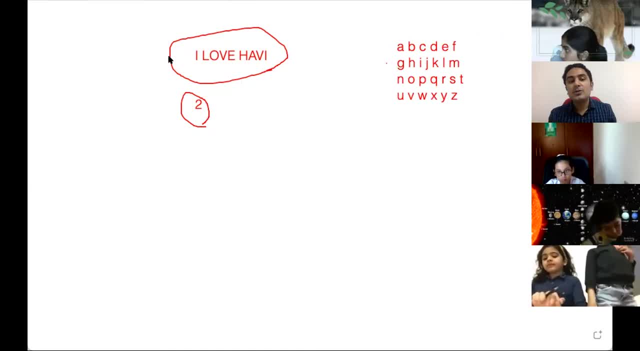 have to jump forward by 2, so i, i is here and jump 2, that means i plus 1 plus 1, that is k. so first letter becomes k. so our cipher, you know our ciphertext, becomes k, then l, so l is l plus 2, that means m and n. so k, n, then o. o is plus o plus 2, that is q. 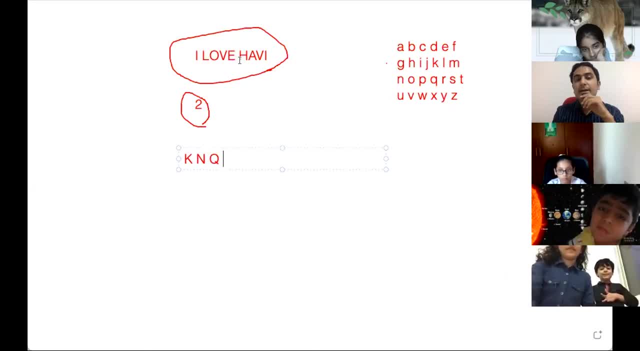 then e, e plus 2, so f and g, that means g. now h, a, v, i, so h plus 2, h, i, that means j, so j, a plus 2, a and b and c, then v plus 2, this x and i plus 2, that is k. so this is our. 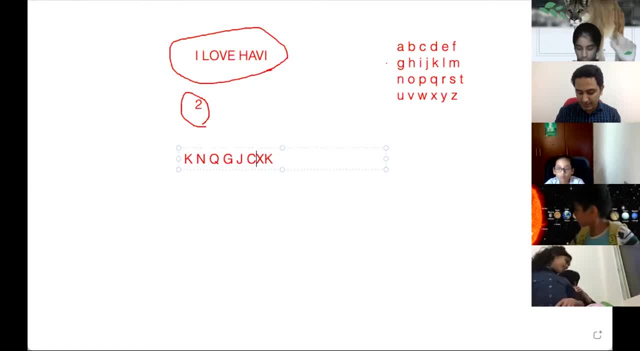 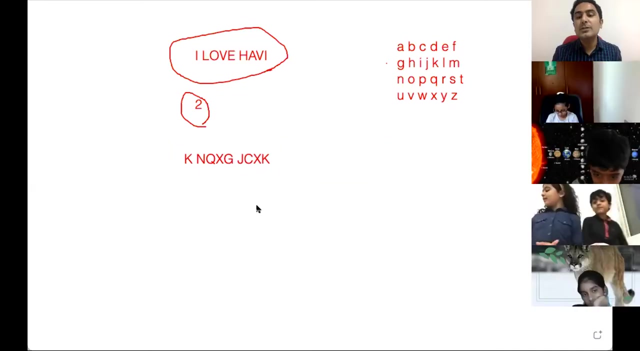 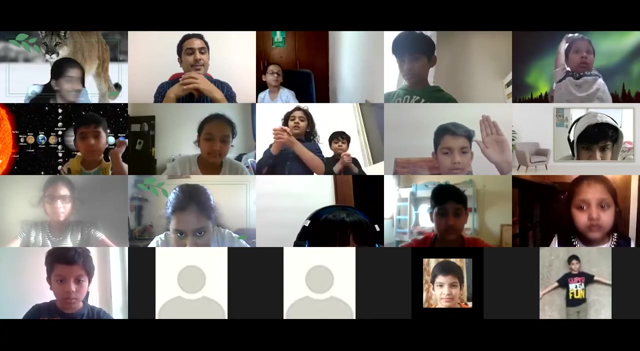 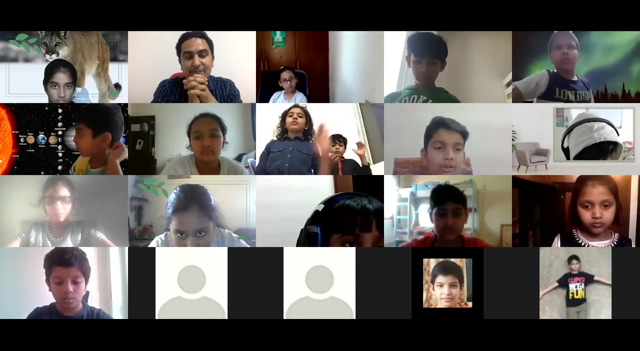 ciphertext, our coded message ciphertext. okay, i think we missed one character, that is l and n. okay, q to q and v to x. yeah, so here is x. so this is our ciphertext. okay, aro seems to have a question. yes, aro, sir, i did it like, instead of doing like. like there's one word and then you do like example. 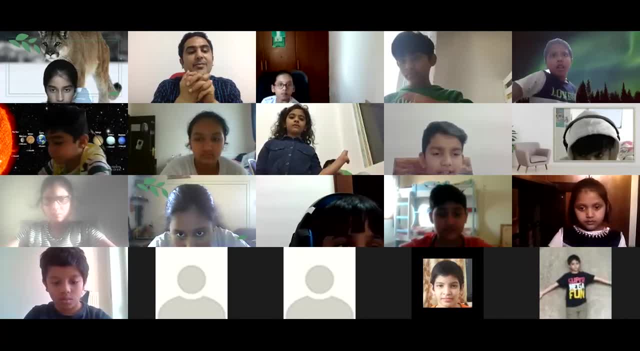 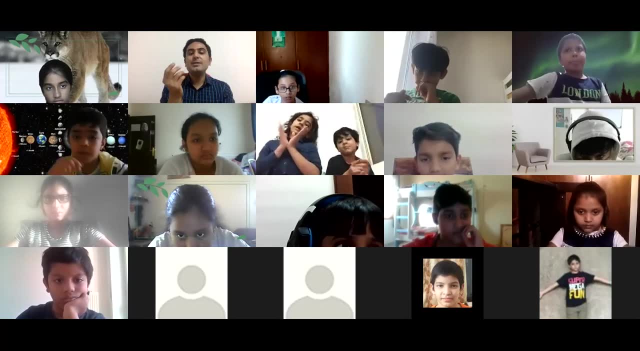 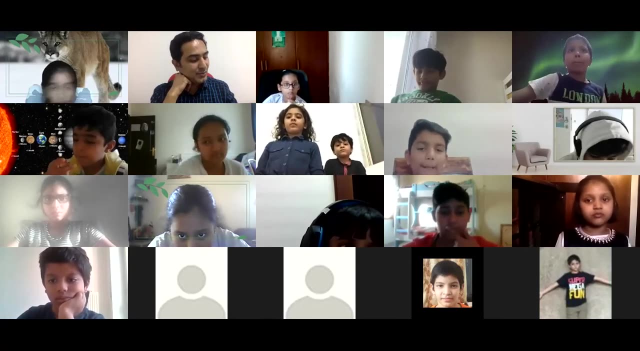 it's h- no example. it's a a- no example, it's a a. then it becomes c. i did like: a becomes y. i went backward, you went backward. so that means the key becomes minus two. right, oh, okay, and key becomes minus two, isn't it? that makes a lot of difference. no, if you're. 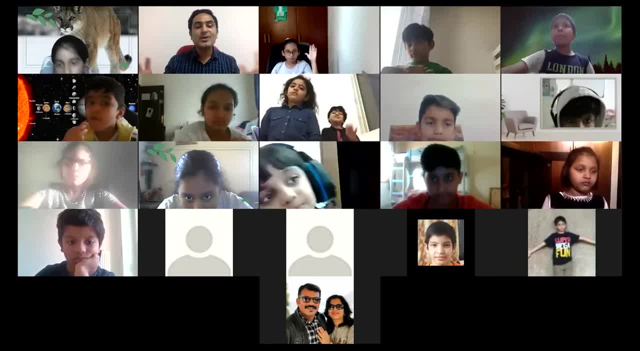 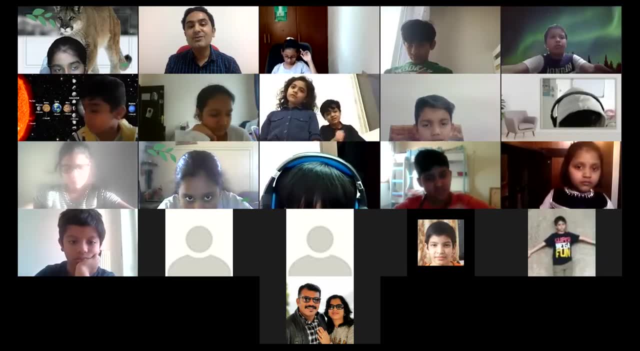 okay and you do minus two, then you will never decode. someone have asked. maybe you know. imagine in the cases of war someone would have asked, you know? imagine in the cases of war someone would have sent a secret message that we have the enemies here. send the support, send the backup. 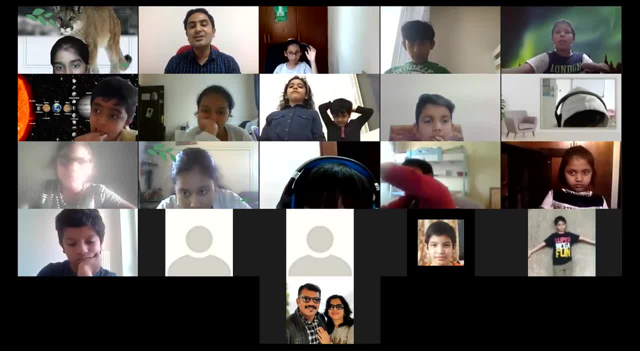 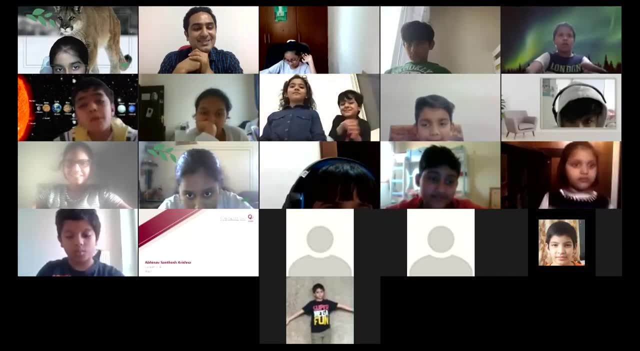 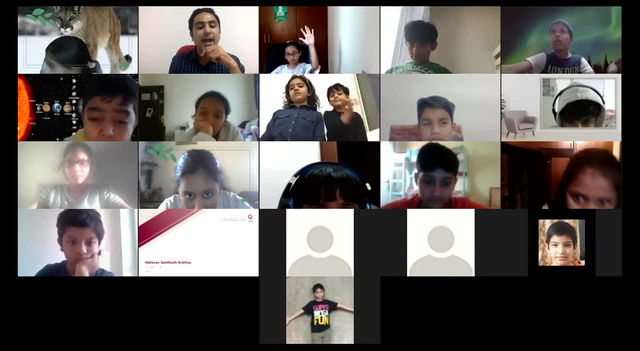 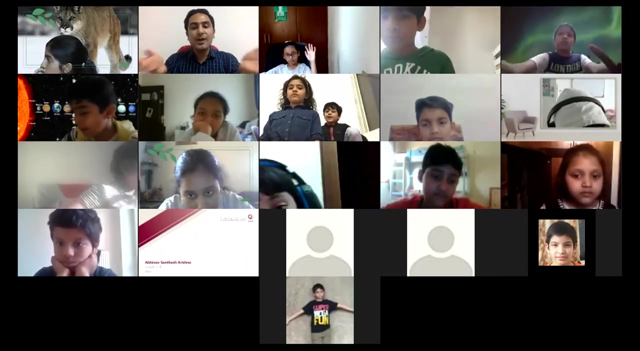 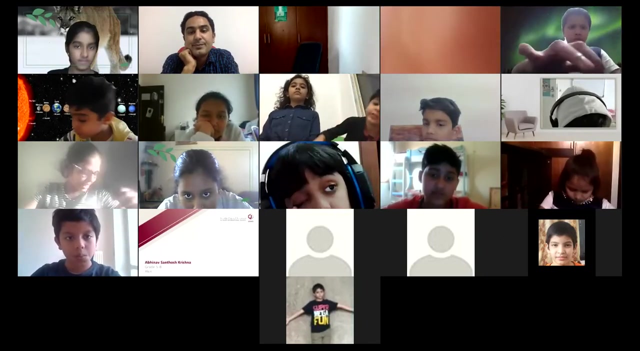 immediately. and what if, instead of two, they use minus two? what will happen? they'll never know what the secret message is. right? okay, so this is ciphertext and plaintext: encryption and decryption and in general, it is called crypto. Now we did this. Any questions so far in this? No, So let's have coding. Do we want to code? 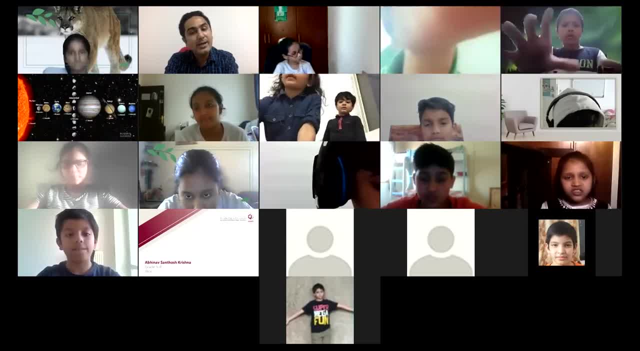 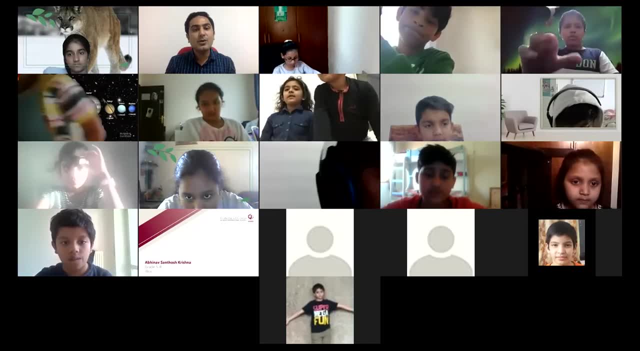 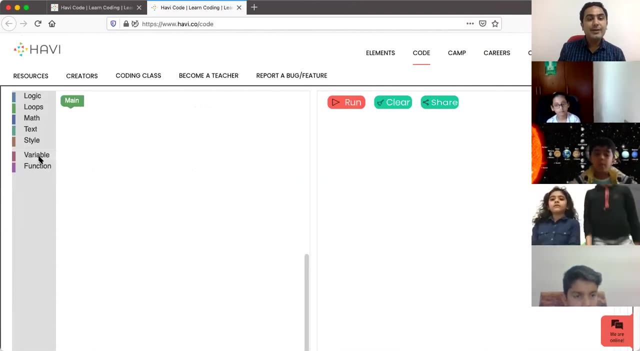 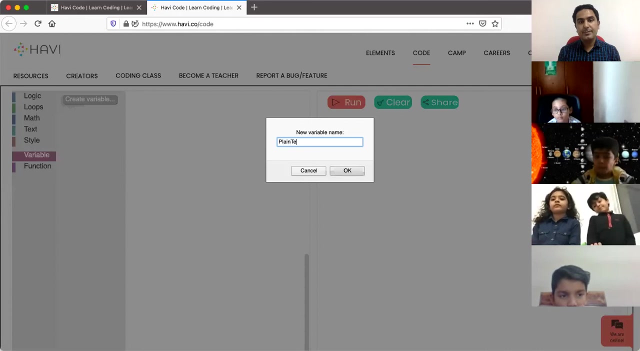 this Shall we write the code to encrypt and decrypt a message. Yes, Let's do that. So we open hubby code. I'll share my screen. So here we create one variable first where we use the word plain text. Okay, We created the variable and then we set a text here. 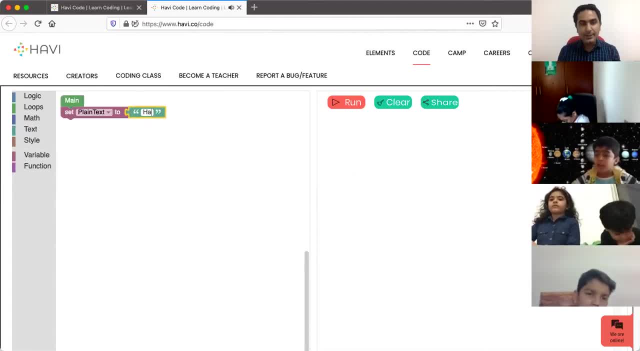 And our plain text is, for example, hubby. Okay, Now, very in the loop. Now, what we need to do is we'll have to add the key into each of the character, Am I right? Let's create a variable Key? Okay, And set key to some. 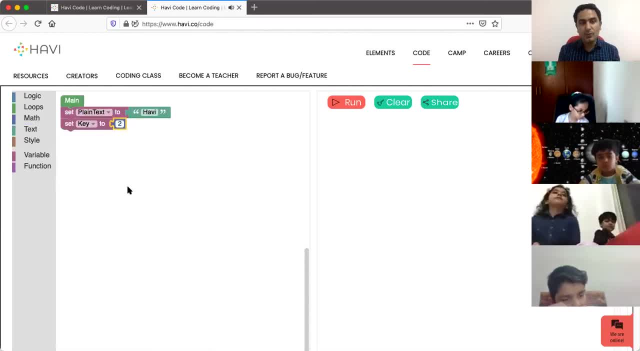 number. Let's say our number is two, Okay, And then we'll have to add the key to some number it to two of these two characters. This some is the key. Now the problem is we'll have to add a two to H, Two to A, Two to B, two to I. how will we do that In coding? 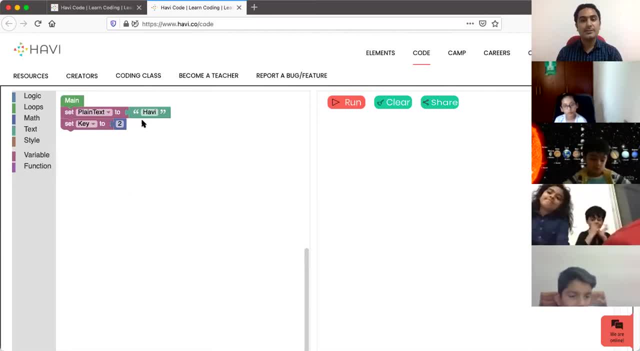 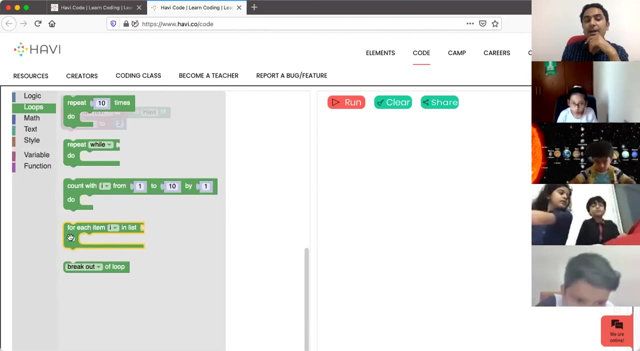 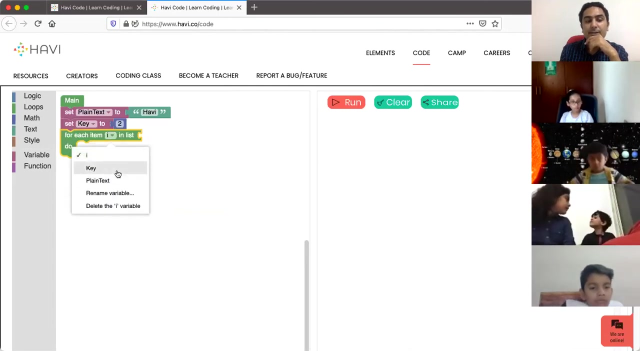 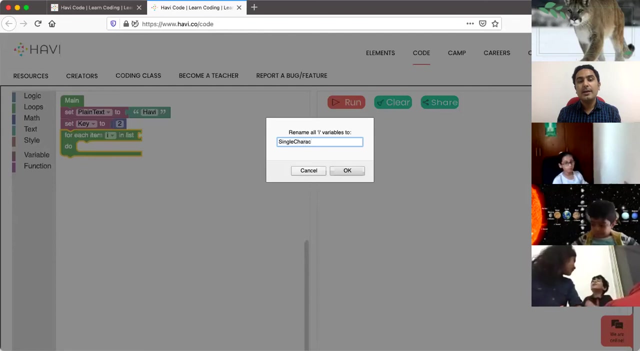 So we'll have to separate those characters, each of them. How will we do that? Well, that got the loops and here you have this loop for each item. i bring this. i will rename this variable i to single character. okay, for each item, that means each single character. 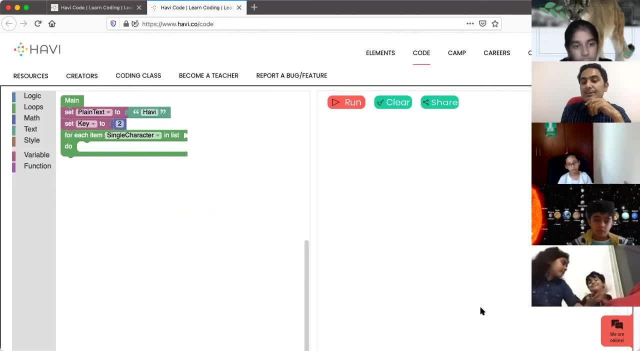 in list. now what is the name of our list? what is the name of our list? it is plain text. our list, that means the list of characters, is stored in the plain text, right? so i add here plain text. here is the plain text now. next we create one more variable, that is: 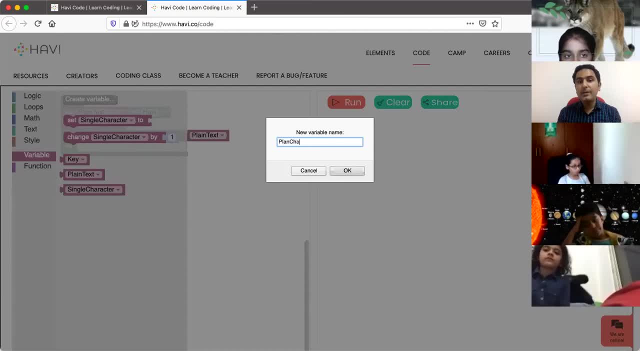 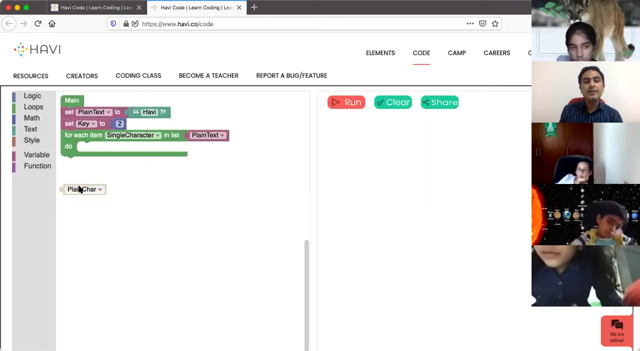 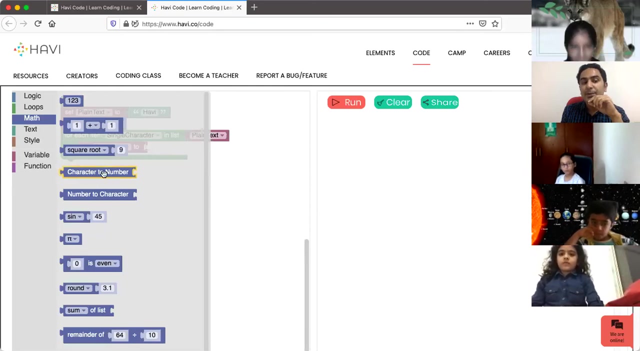 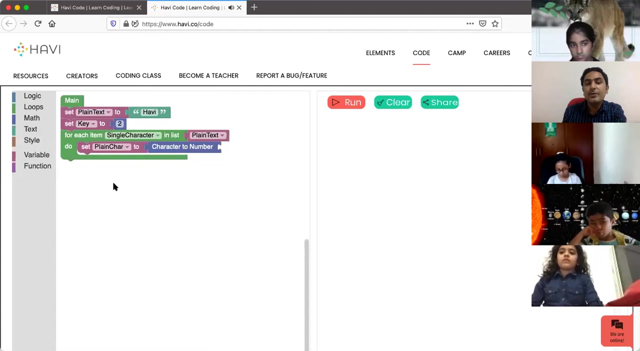 this plain character. i am just writing short c-h-a-r plain character. yeah, it should be plain character, not planned character, plain character. so here is the variable: plain character. i will set that plain character. okay. Now here is the important thing. Go to math and there you find a command: Character to number. Character to number, That means it converts your character into a number. So character to number and what you want to convert, This single character. 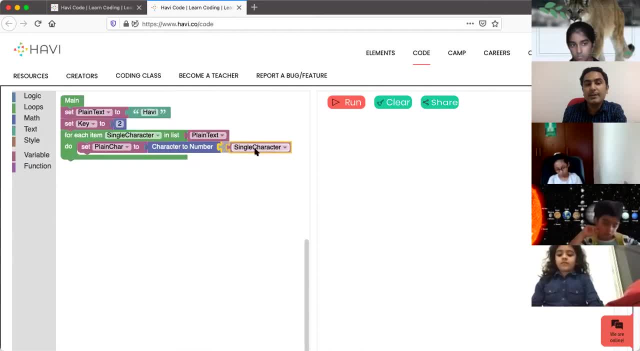 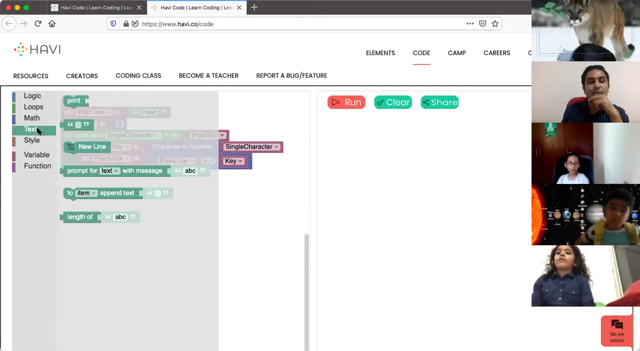 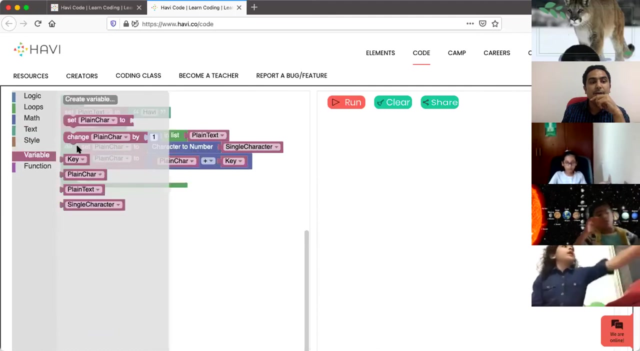 So variable single character. That means convert single character to number and give that to plain character. Okay, And then variable set Plain character, Math, and add your key, Plain character plus your key. Okay, So now we have the plain character with key. That means encryption is done. Now let's again convert character to a number to character. This is number. at present We can use this: See print: variable plain character. 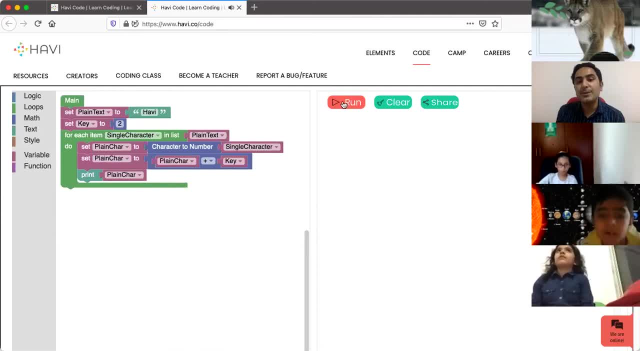 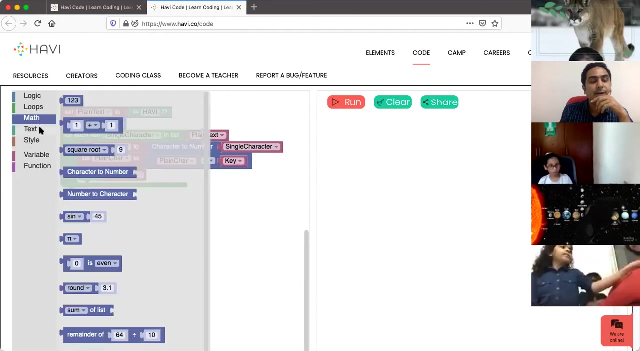 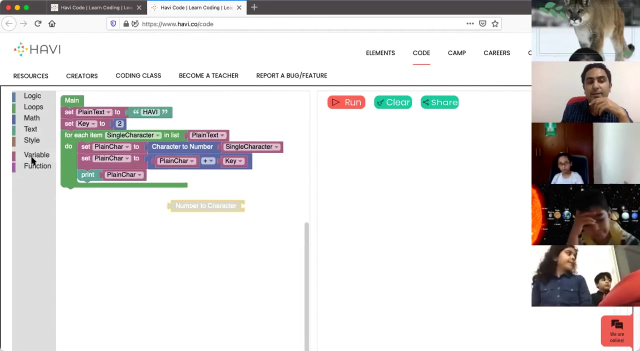 If you print this and you will see what happens. See, now, these are numbers. It is converted into number. Okay, Now we want this to again go back to character. Let's do that. Okay, Let's do that. Go to math, Number to character. So for that we again will have to create a variable. 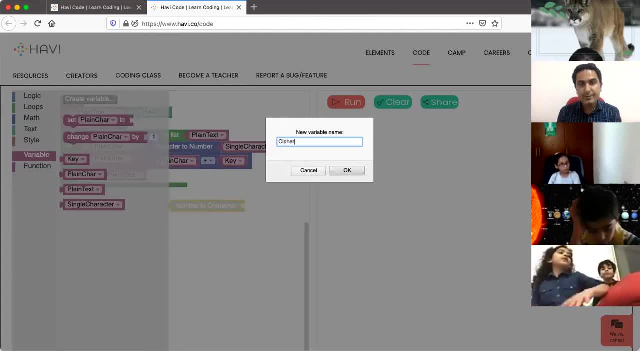 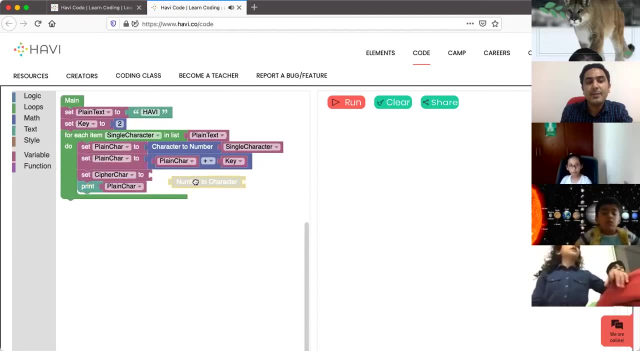 Cypher character. So set cypher character to number to character, Plain character. That means convert your plain character to character again. This means number to character, again with cypher, And then print cypher And you see, This is encrypted now. 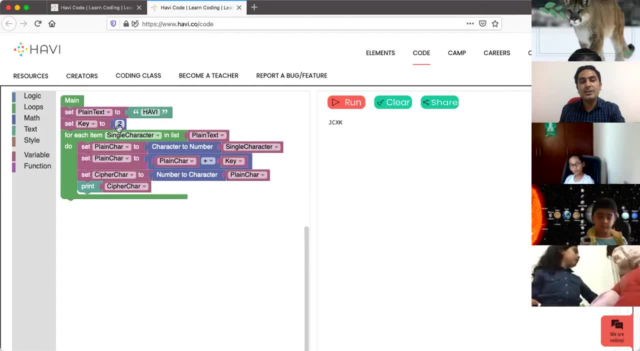 Havi is encrypted to jcxk. If I change the key to 1.. Run ibwj. If I change the key to 0. That means no addition, It's back to Havi. If I change it to 3.. 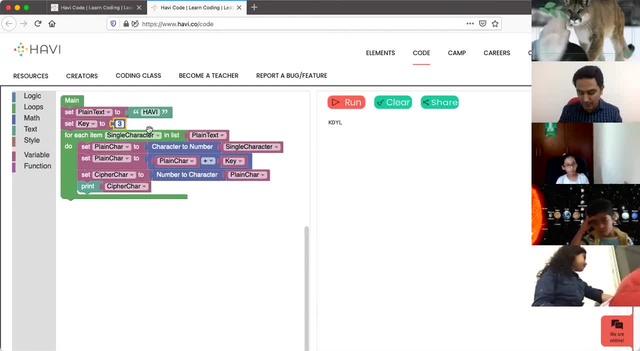 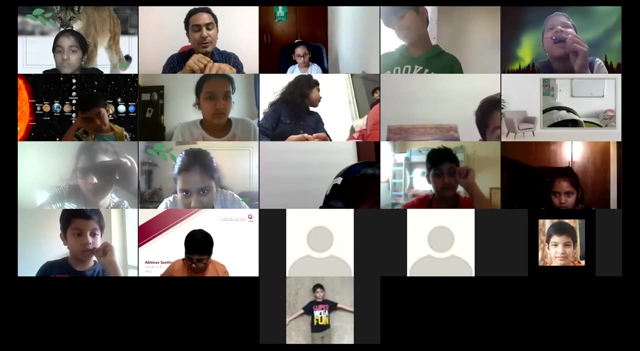 This is secret code. If I convert it to minus 3.. Then something wonderful. See this. Okay, One instruction: When you are using these commands- Number to character and character to number- You will get some special characters. That means you will get the dollar sign. 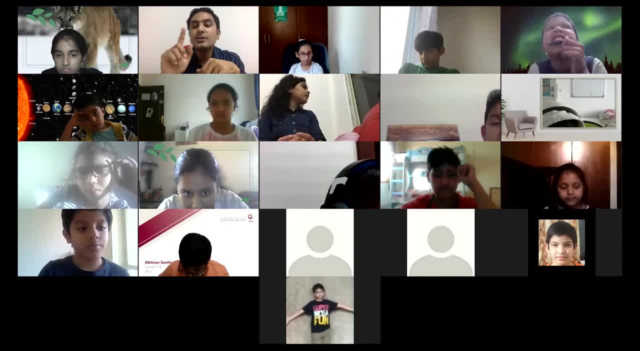 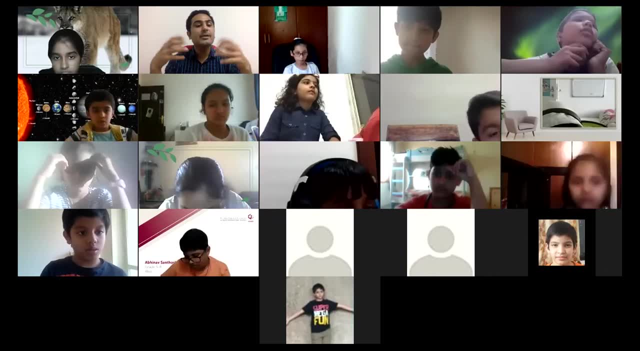 Percentage Less than Greater. than Why? Because these functions are coded for a longer series- Small case, Upper case And many other characters. So you will get those, Don't be afraid about that. Maybe somewhere in the later class. 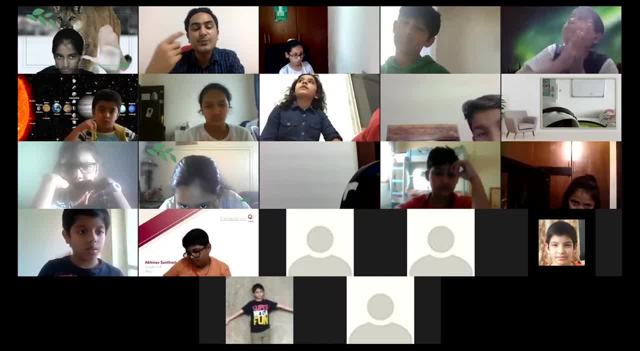 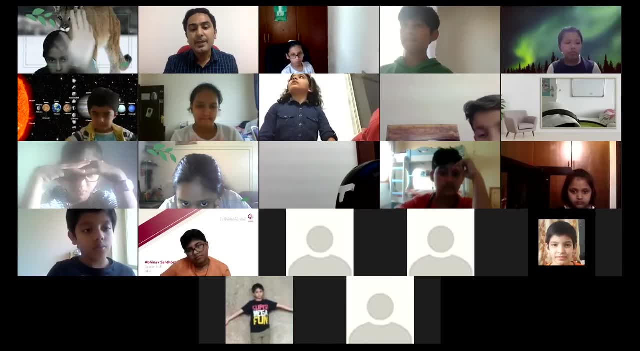 You will learn about that as well. Okay, Why those special characters are coming up For now? Just consider those. Is that clear One thing? If I, I will share the screen again. See here: The key is 3.. 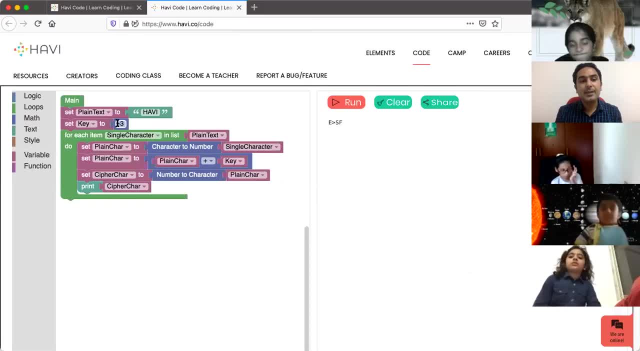 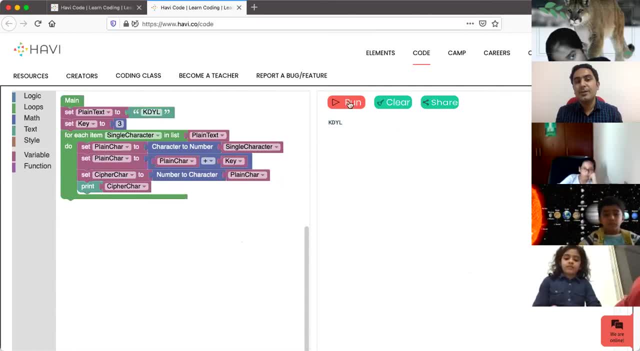 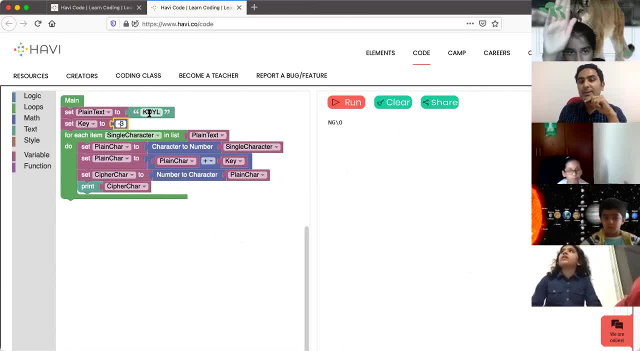 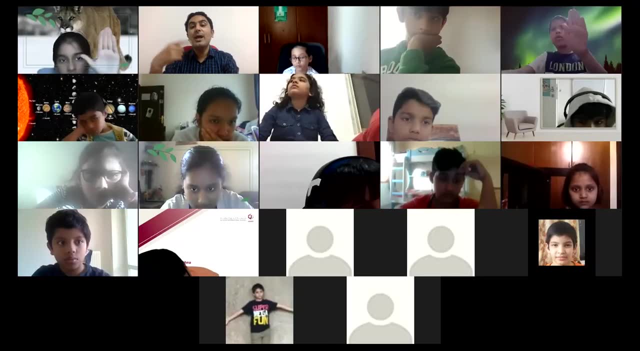 From plus 3. To Minus 3. Can you tell me What will happen now? Here In the plain text I have put The secret code And the key is minus 3.. Show me your hand If you can tell me. 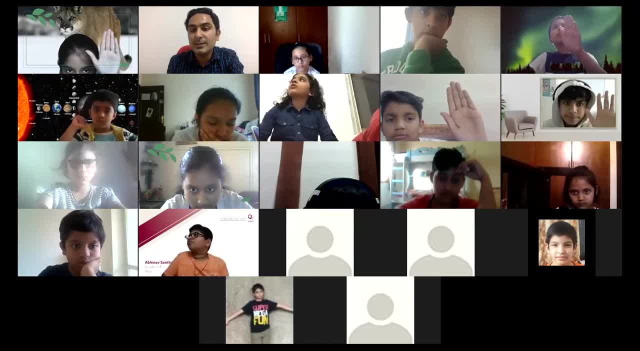 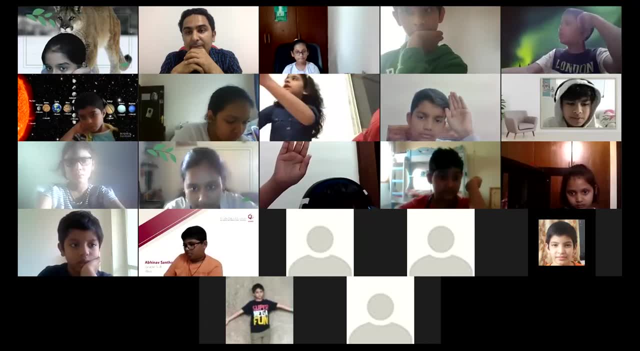 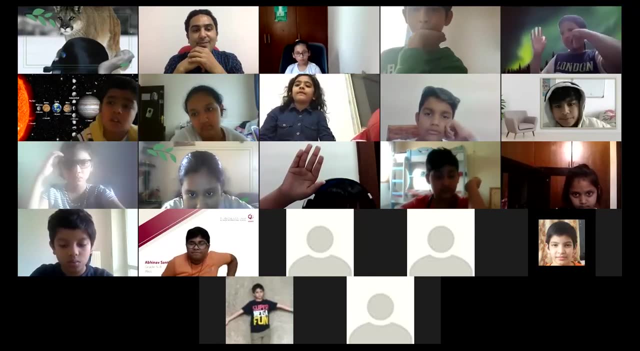 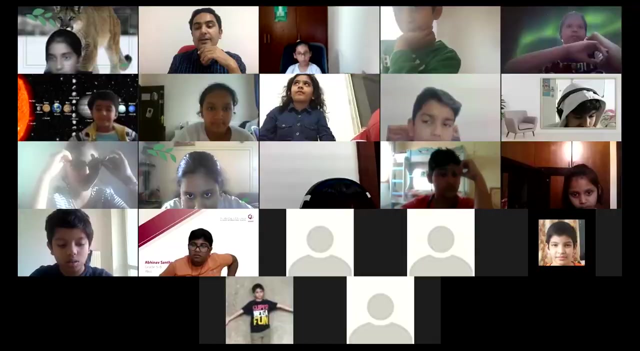 What will happen now? What will be the answer? Yes, Kahan, You want to say something. You want to answer Okay, um, it will be back to hubby. very good, it will be back to hubby. so that is decryption. okay, nice, so that is the encryption and decryption now. 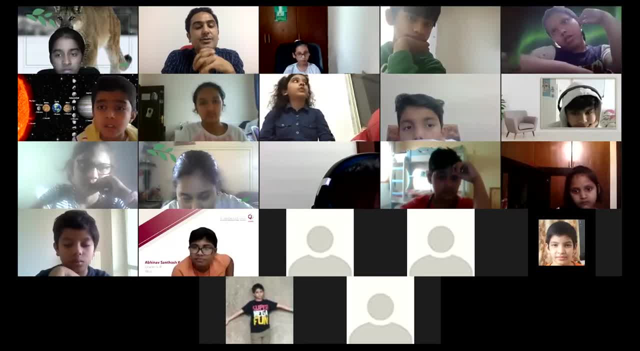 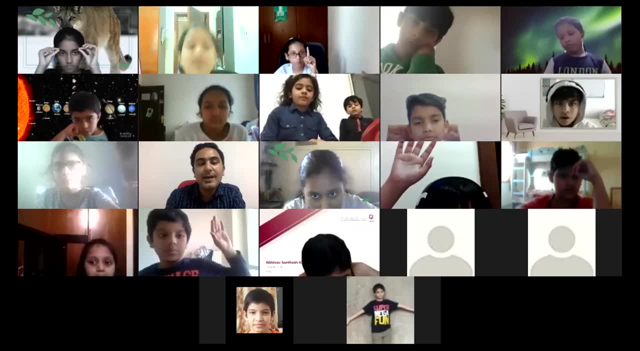 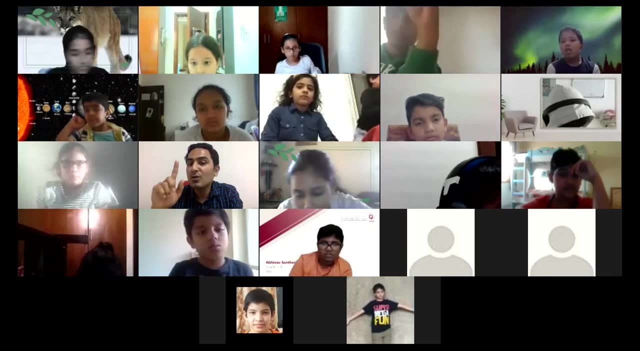 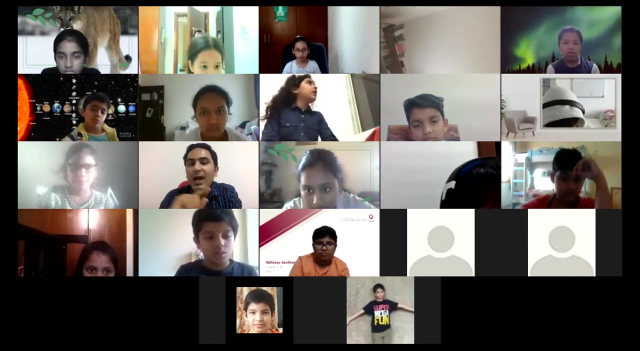 i have a challenge for all of you. who wants to accept the challenge? i will write a text. i'll write a text and you will have to write the code. you will have to. i will not give you the key. i will write the cipher text. i will not give you the key. 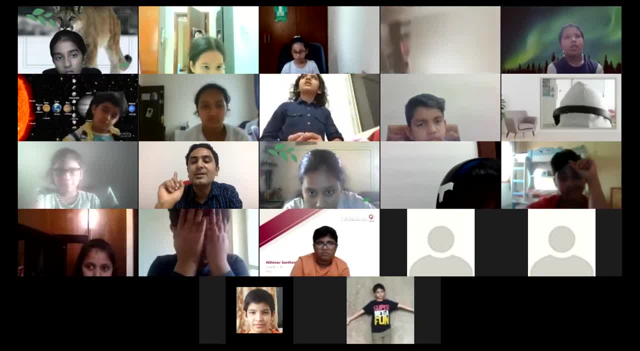 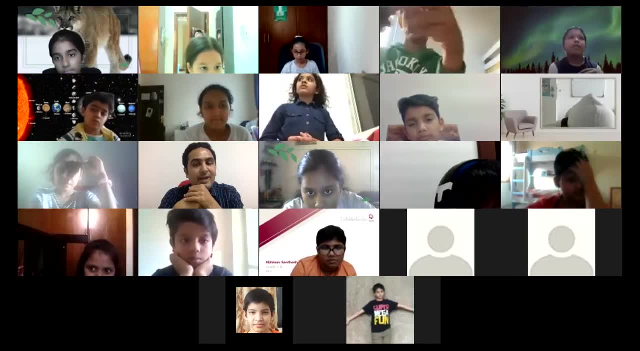 you will have to message me the plain text after the class. that means you will have to write the code yourself and then i will write the code for you, and then i will write the code for you. try various key. okay, is it one? is it two? is it minus one? is it minus two? what? what is the key? 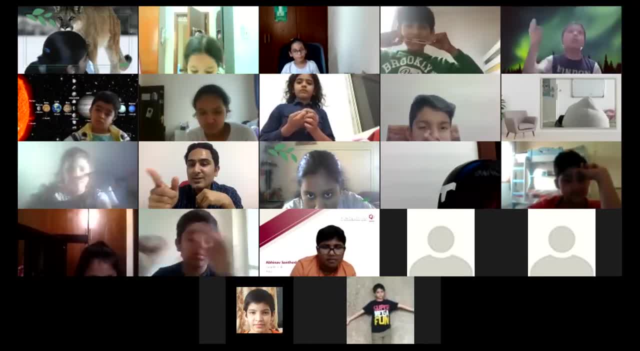 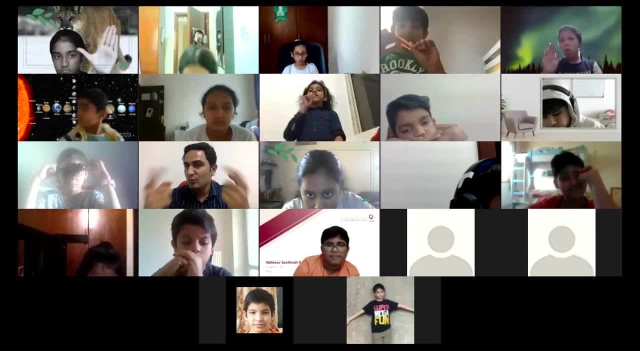 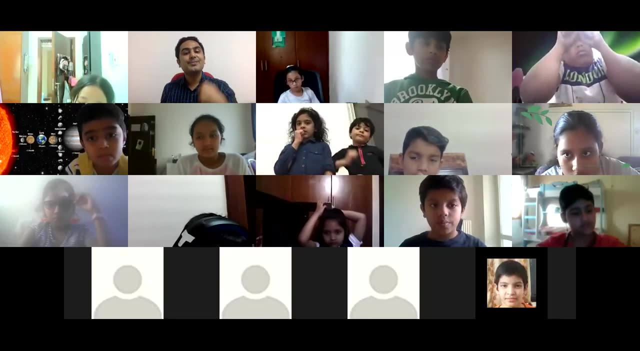 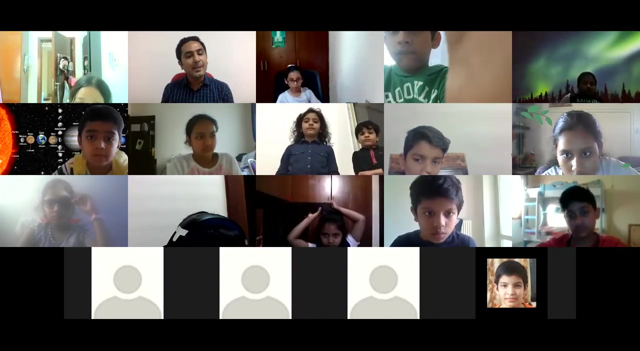 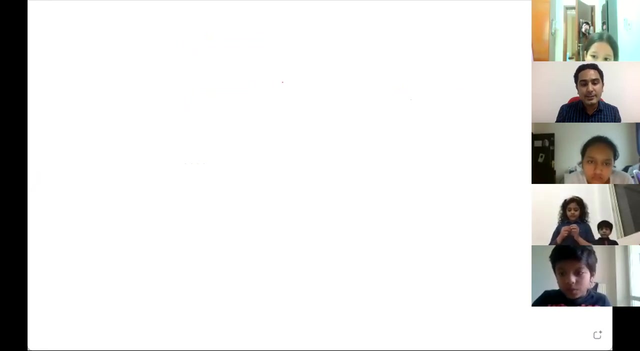 try various key and you will find out if you can understand the message. that means that is the key. so send back the key and the plain text to me. is that clear, understood? share your key and write message with me on whatsapp or email. send me email on cam at hubbyco or the whatsapp number you already have. so here is the key. so the text is: 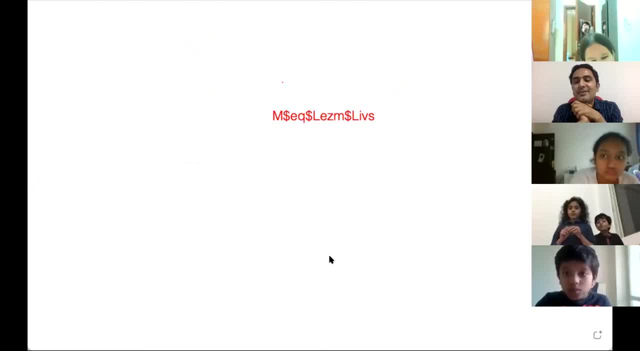 this: okay, this is the text. this is the cipher text. you need to enter the cipher text and write the key. you will have to write the code. try the keys and then send me the message. send me the key, okay, bye.